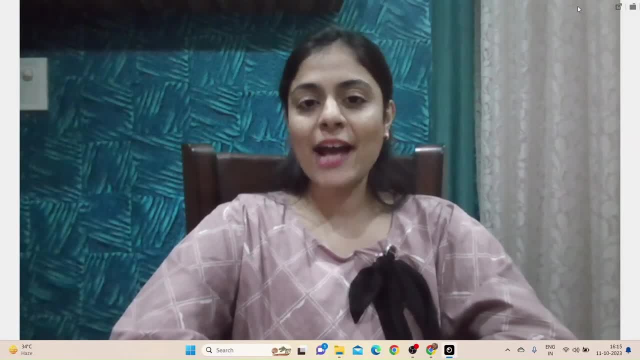 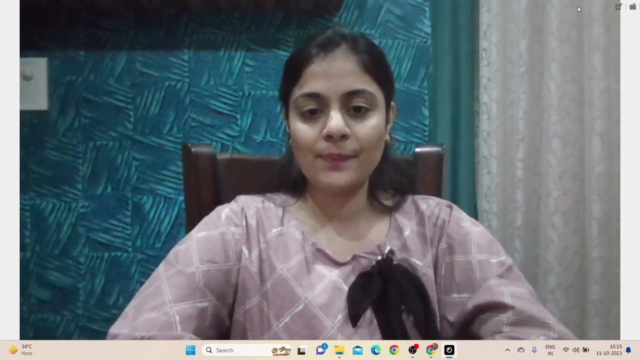 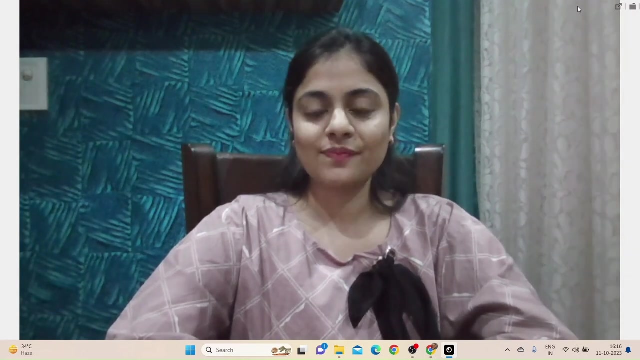 hello everyone and welcome. I am Pratibha and I am a machine learning engineer at ProDesart. in today's video, we will explore an exciting machine learning project, or more precisely, a natural language processing project. our focus will be on named entity recognition, which is commonly referred to as NER. so 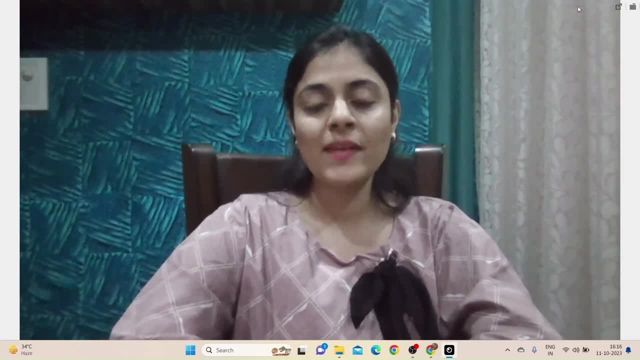 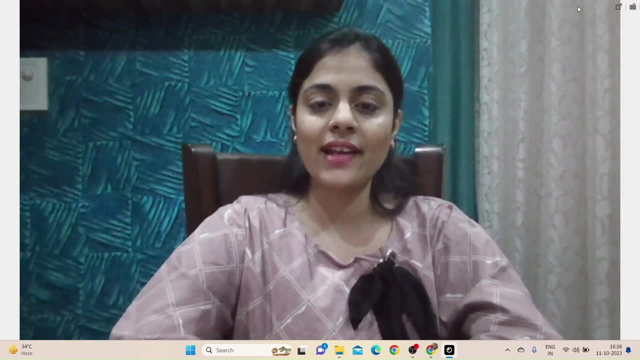 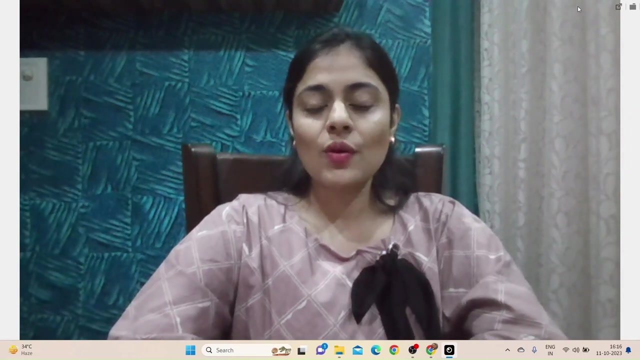 let us first try to understand what is NER. named entity recognition is a subfield of NLP which deals with identifying and classifying named entities in text. data and named entities are nothing but a real world objects like people, organizations, locations, date and so on. so NER plays a crucial role in information extraction and 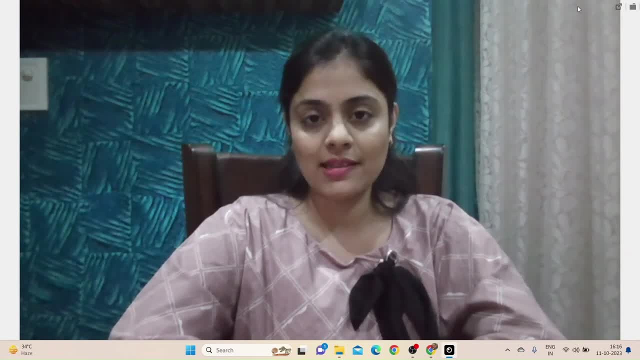 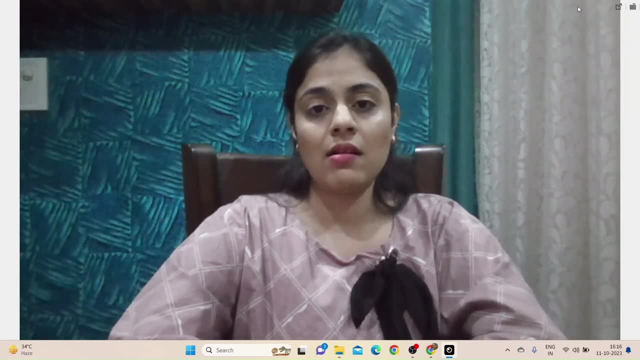 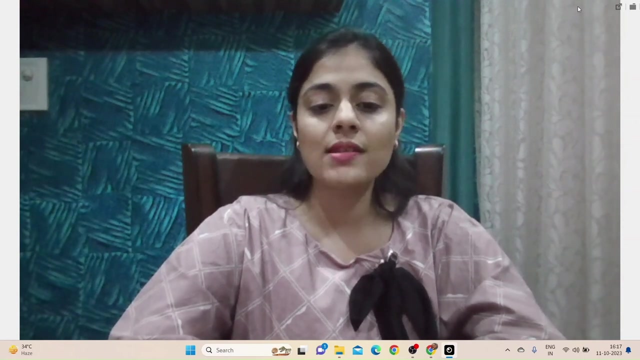 understanding the structure and content of text. now it has a wide range of applications. it has found its use in information- Katy Evaristo, Oral Idea of Abrtln and search engines, in social media analysis, in medical health records and healthcare analysis and legal document analysis. also construction document analysis. like it is, its uses can: 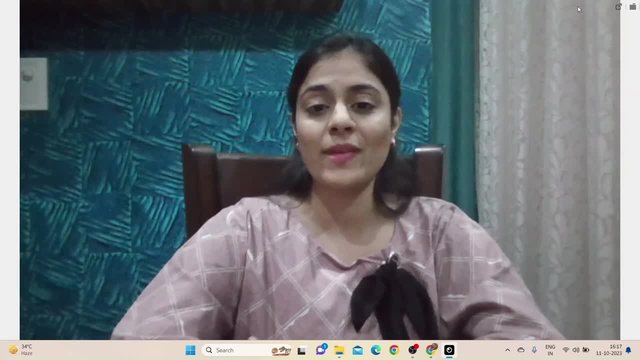 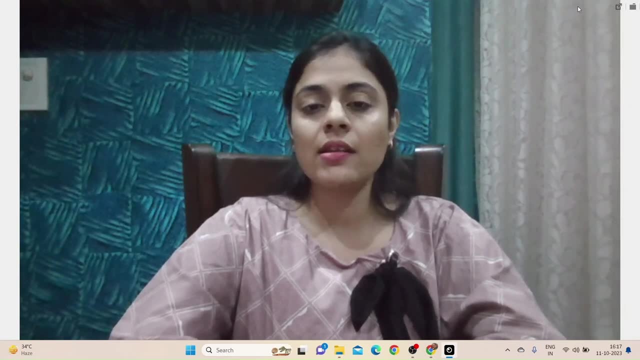 be found in various industries, documents related to various industries right, and if I am to elaborate more on it, then in information retrieval, NER helps search engines to understand user queries and retrieve more relevant results, and in social media analysis also, NER is particularly used for sentiment analysis only, and in there NER can help to identify entities that people 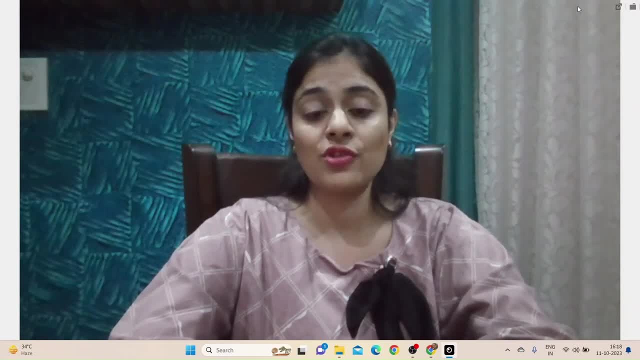 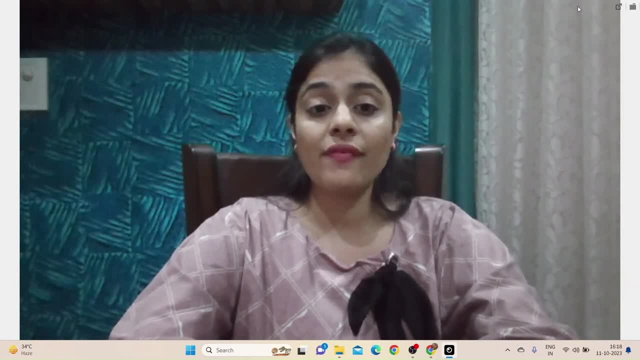 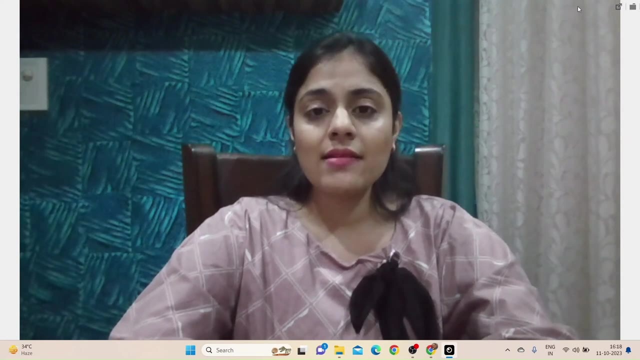 So let's move on to the next slide. Also, we can find the use of NER in content categorization. it can be used to categorize news articles, social media posts and various documents based on the entities that are mentioned in them, and, moreover, it has also found its uses in chatbots and virtual assistants, where 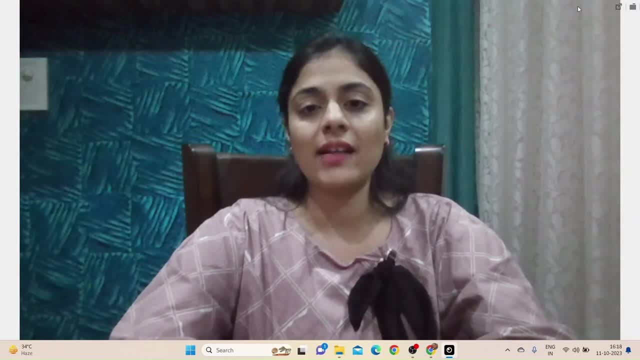 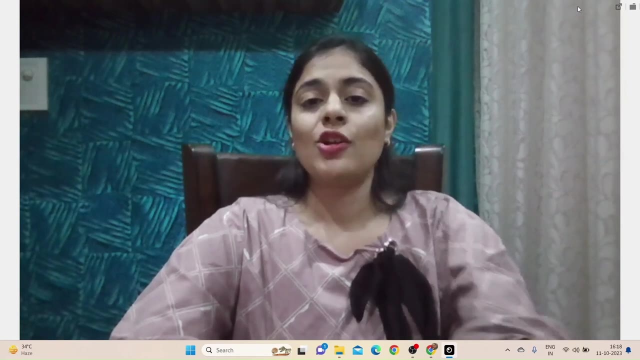 NER can be used to identify specific entities mentioned by the users to provide relevant responses. So you can see that the use cases for NER are many fold and that is why it becomes extremely important to learn how to implement NER. that is named. 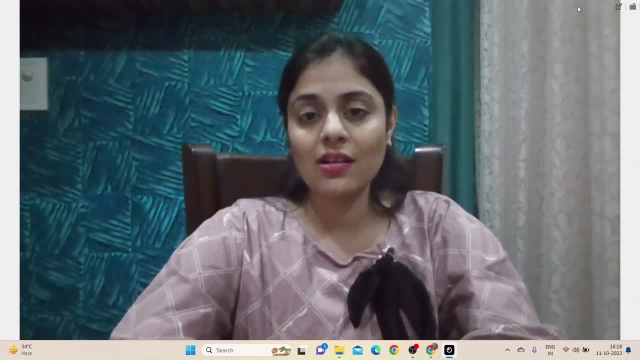 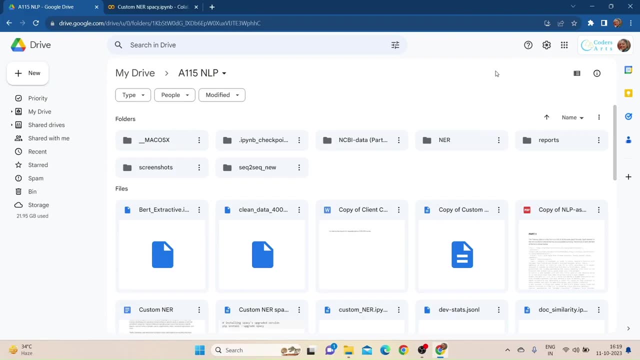 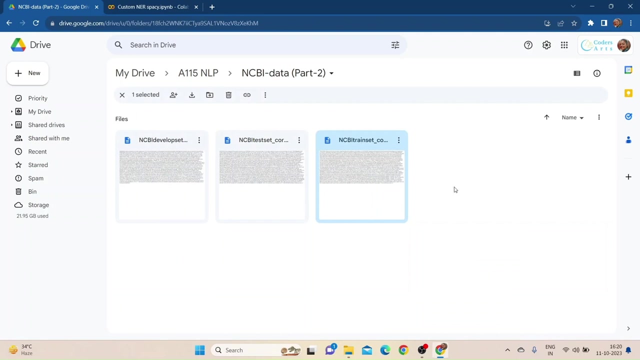 entity recognition and train NLP models for the same purpose. So let's dive straight into the code. So on the screen, you can see a Google Drive folder where our training data and the testing data is present. The training data is provided by NCBI and let's just quickly take a. 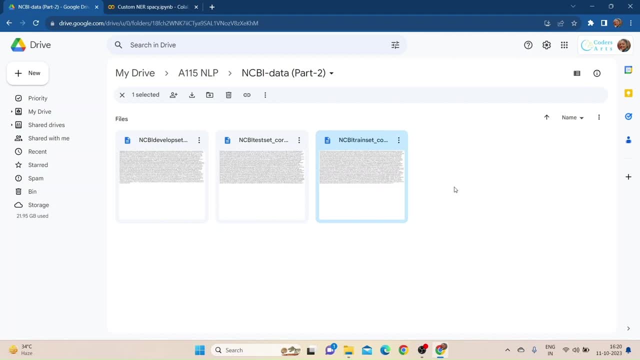 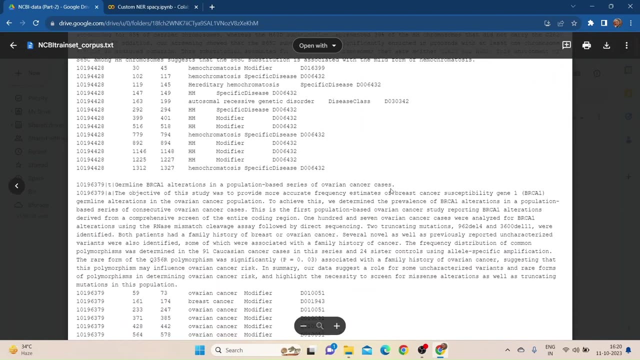 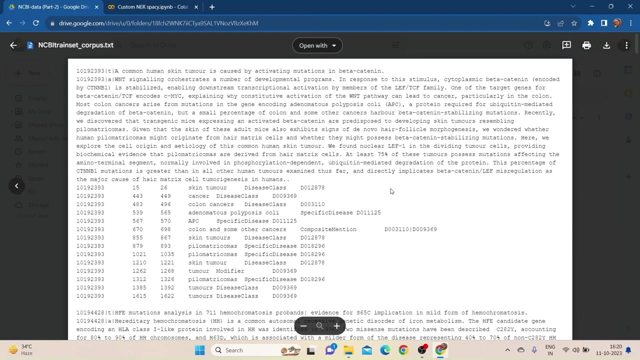 look at the training and the testing data, because it is a good practice to familiarize yourself with the data that you are working on and understand its structure. So this is the text file containing the train set and you can see that it is following a particular structure. Let's just try to. 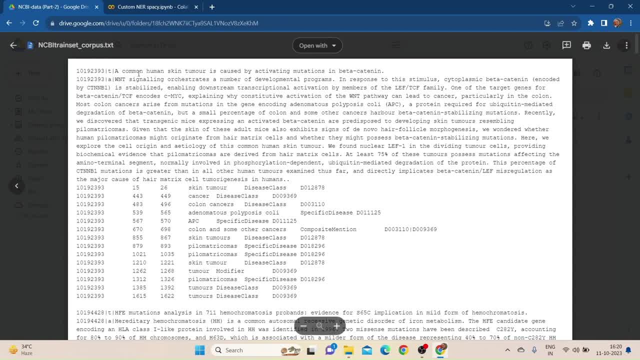 understand what it is. So here between the pipe signs, you can see that a letter T is present and it basically corresponds to the title of the medical text that we are seeing here. So this particular line is the text, and then again in between the pipe signs, there is a letter A. 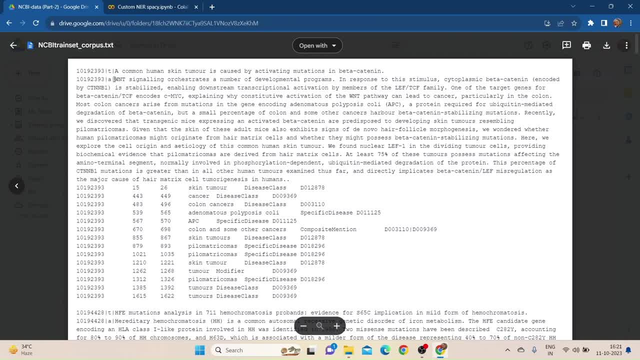 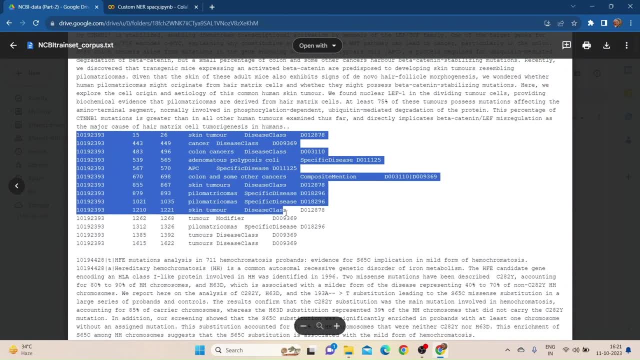 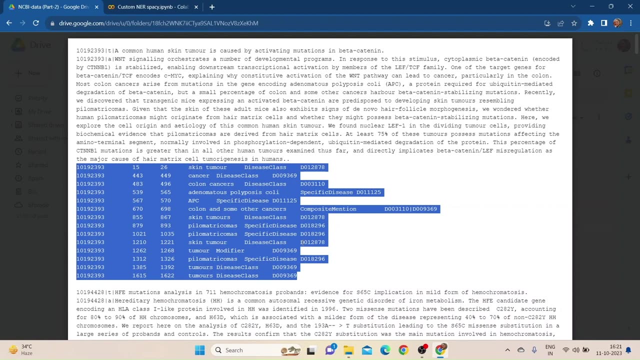 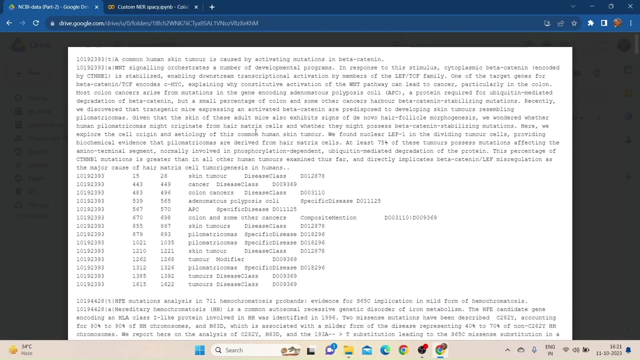 That represents the article or the body of the medical text. So this is the body, and then we have some tab separated text which you can see that appears to be like a table right. So this is the annotation of this text. Now, one thing that you need to understand is that the annotation here 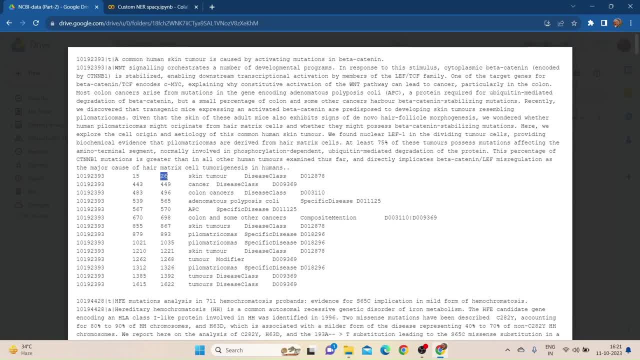 represents the indexing of the medical text. So this is the annotation of the medical text, So this is the text and then again it is the title of the medical text. So the annotation of the medical text is represented by some of these two words right, And this indexing is being calculated from. 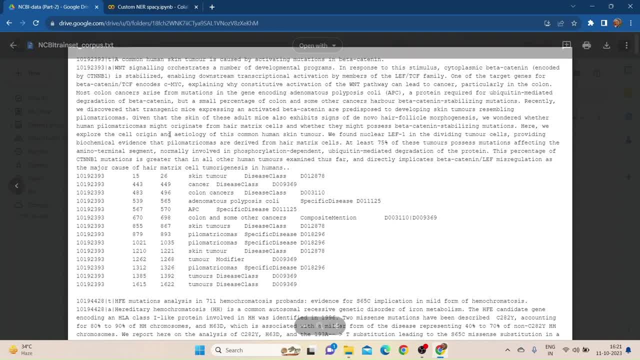 the title itself. So the text that we are going to focus on is not just the article text, but also the title as well. So the concatenation of the title and the article provides us with the medical text that we are interested into, and these numbers here are nothing but just the Id of the. 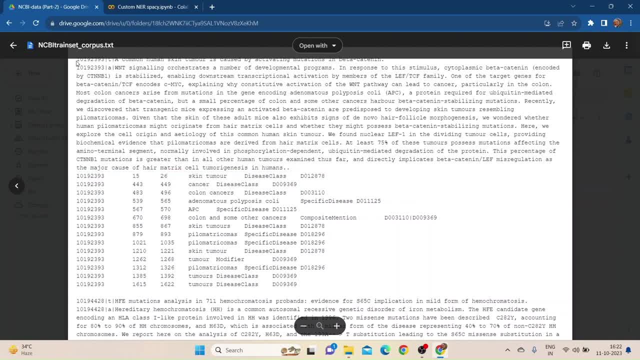 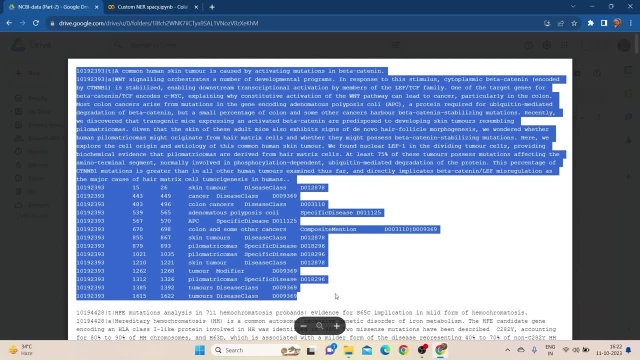 instance of the data. for example, from here, from this point to this point, we have one single instance of the data in our training set and you can see that the id remains the same for that and basically the purpose of the id in the train set is for this, only for this kind of indication. 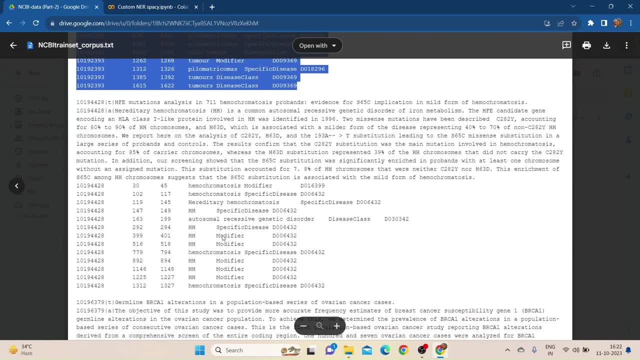 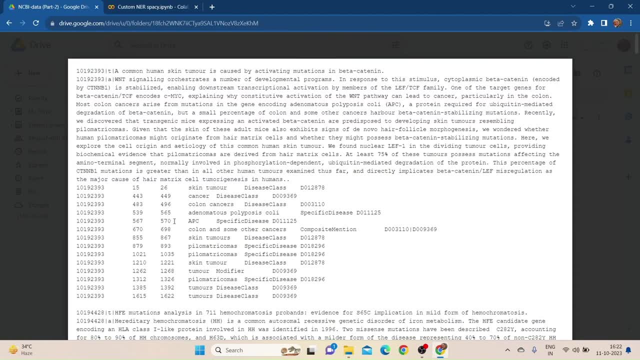 and then here we have another instance, and then another, and so on. so for all of them we have a title, an article, and then the annotation. now let's just quickly try to understand what this annotation here represents, as i have already told you that this is the starting index and this is 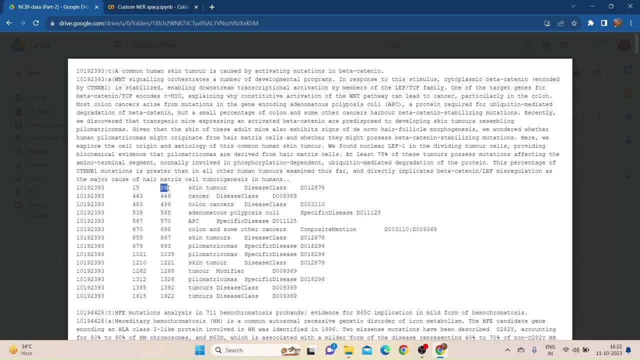 the ending index of a word, and that word is mentioned here, that is skin tumor. now, in this particular text, when we are like starting the index from the title, that is, this letter a is a title, and then we have a title, and then we have a title, and then we have a title, and then 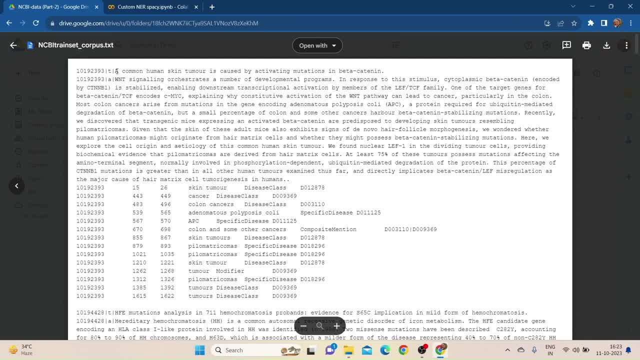 at the position zero. okay, so with this kind of referencing, if we calculate the 15th position, then it will land on the s letter of the skin tumor. you can also verify it right here from the text. you can just directly count it. let me just do it for you here. a is at zero, then we have 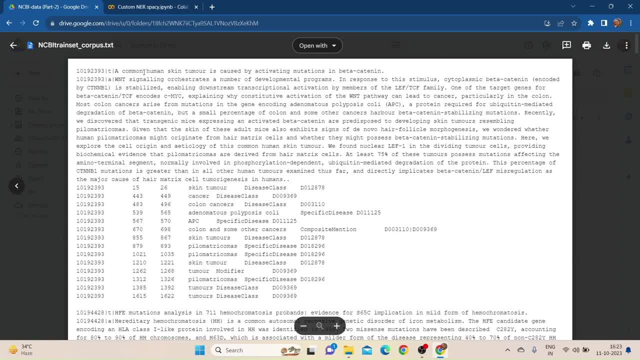 1, 2, 3, 4, 5, 6, 7, 8, 9, 10, 11, 12, 13, 14, 15 and 15. as i told you that the 15th, the letter that is present in the 15th position, is the letter. 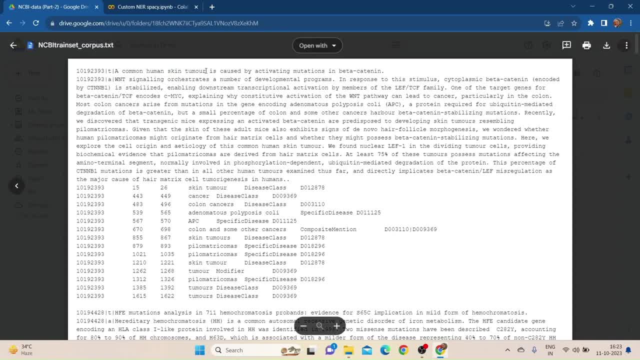 s from the skin tumor, and this space is being represented by the position 26, and then if you take the text from the title into a string and you try to extract the substring, which is ranging from the position 15 till the position of 26, then you will find that you will get this particular 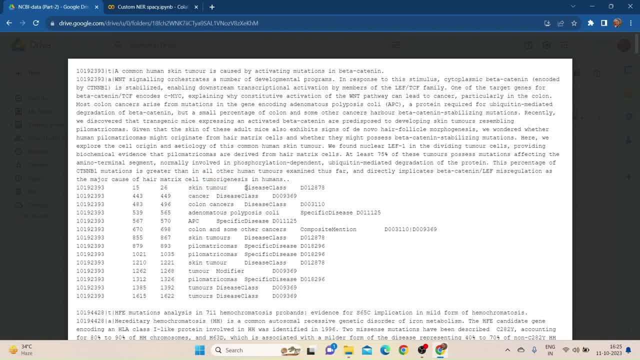 word, that is skin tumor, and then here this word represents the class or the entity to which this particular word belongs to, or the entity which this word is representing. okay, so this skin tumor is a disease class, so you can think of it as a category or the entity for it. and here this is the. 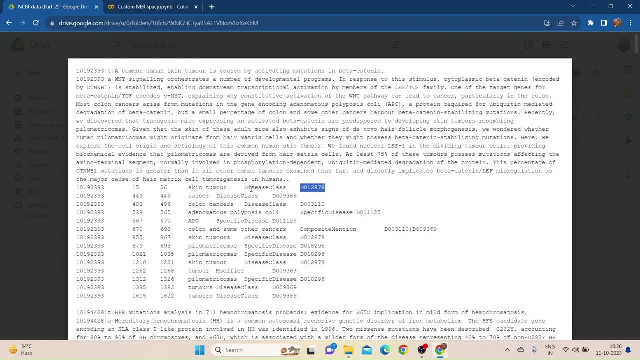 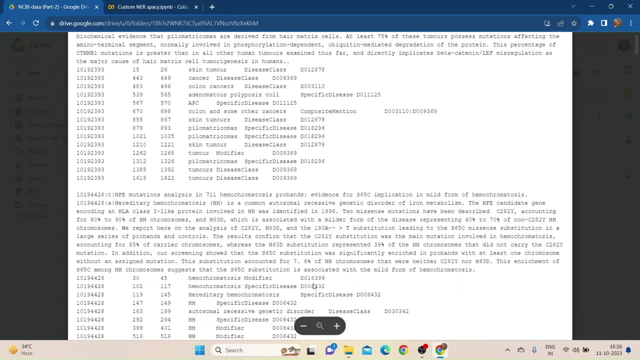 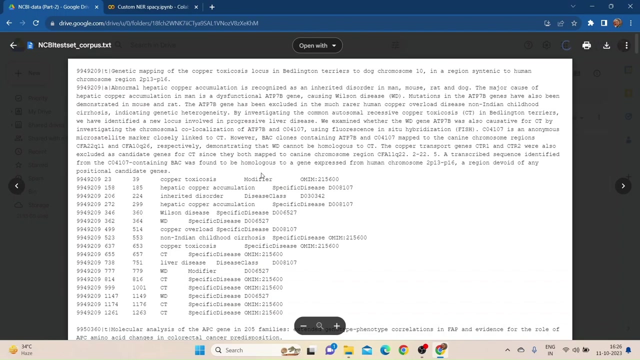 code for the entity. okay, so disease class is being represented by this code, as you can see here later on also in here, that a disease class is being represented by the same code as in here. so that is the structure of our train data, and let's just take a peek at the test data as well, right so? 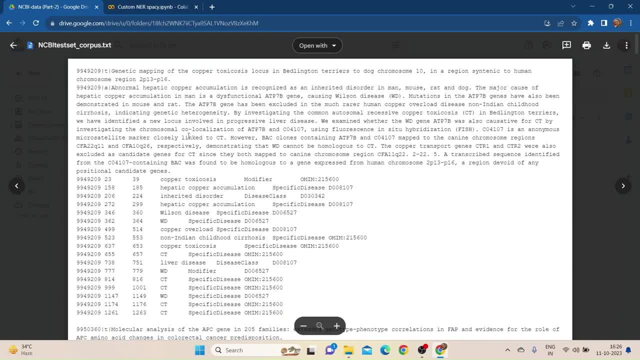 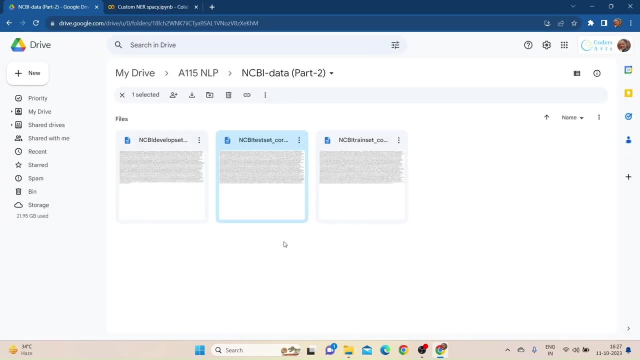 this is following the same kind of structure. we see that the test data is also having the annotation in here. this will help us to cross check the predictions of the model against the original data. so now that we are familiar with the structure of the data, we are ready to move on to the code. 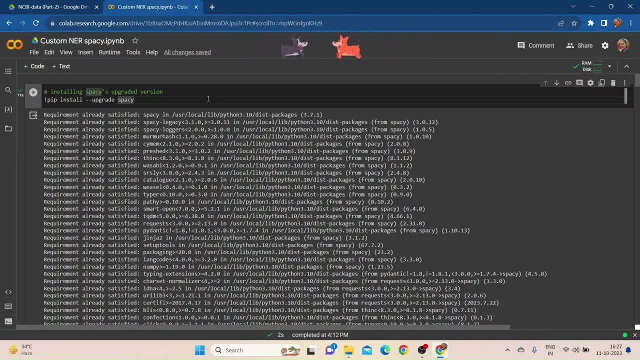 so here you can see in the first line of the code that we are installing an upgraded version of the spacey library, right? so we are going to make use of the spacey library to perform custom ner and spacey library is going to be used to perform custom ner and spacey library is going to 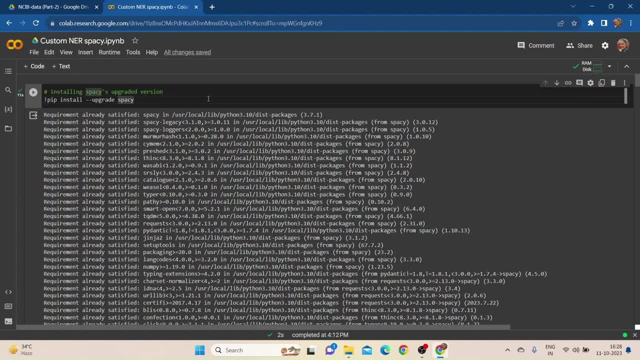 be used to perform custom ner and spacey is an open source nlp library and framework for python. it is designed to help developers and researchers to work with human language data more efficiently and easily, and spacey provides a wide range of tools and resources for various nlp tasks making 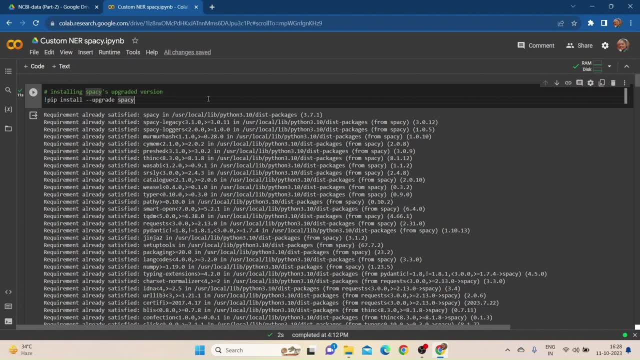 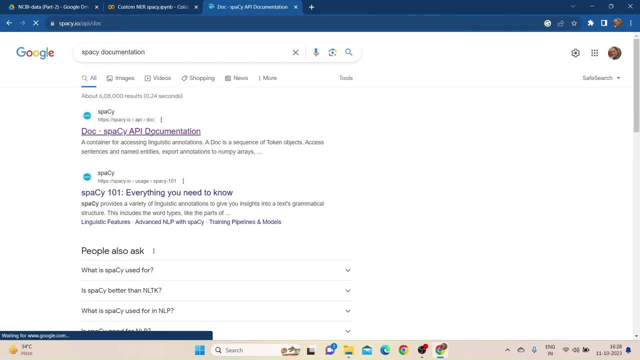 it a popular choice for tasks like a text preprocessing, text classification, named entity recognition, part of speech, tagging and more right. so now let's move on to our next step in this talk. So let's just quickly take a look at Spacy's documentation page. Here you will be able to see different pipelines that are available. 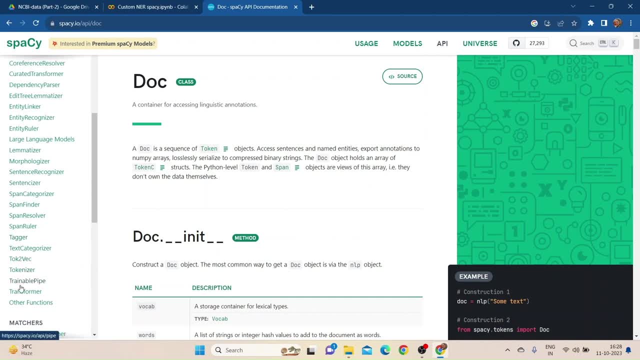 You can see there is a tagger, there is a tokenizer, various transformers are also there. We are going to use a transformer ourselves And then here you can just check out the documentation page to get more information regarding this library. Okay, so let's come to the code. 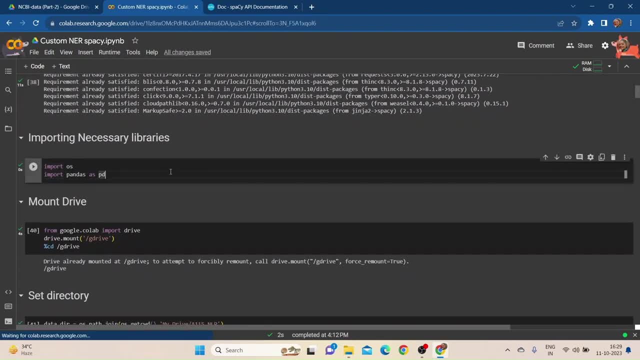 We have imported a few necessary libraries here, But please note that throughout the length of this project, but please note that throughout the length of this Jupyter notebook, we are going to import various libraries as and when required. After that, here we are mounting the Google Drive. 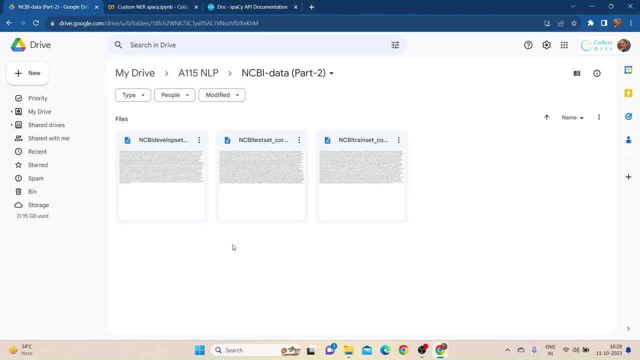 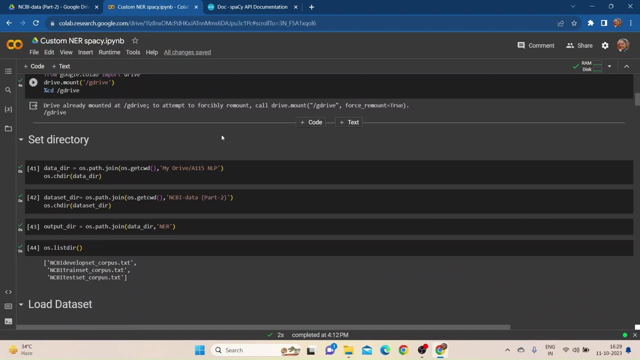 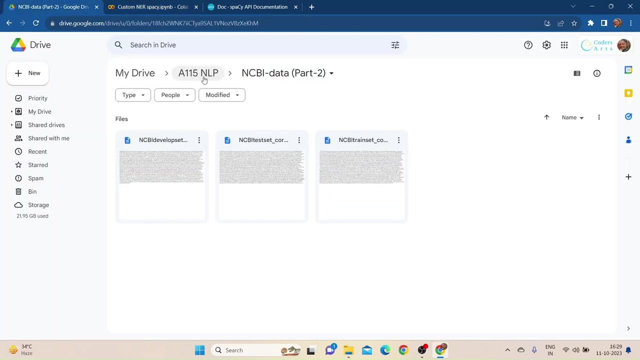 This is very necessary so that we are able to access the database. This is the database data which is present in the Google Drive folder, And after that, here we are setting a path to a few directories. This data directory is basically the path to this particular folder in my Google Drive. 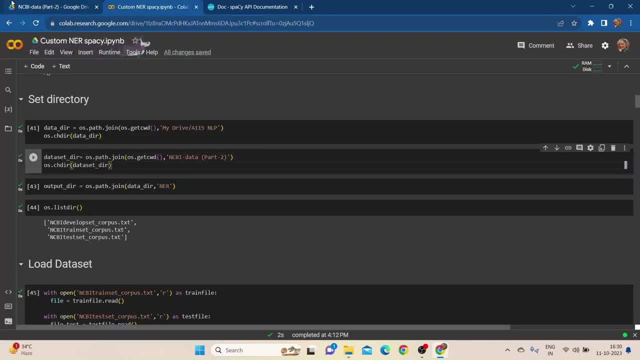 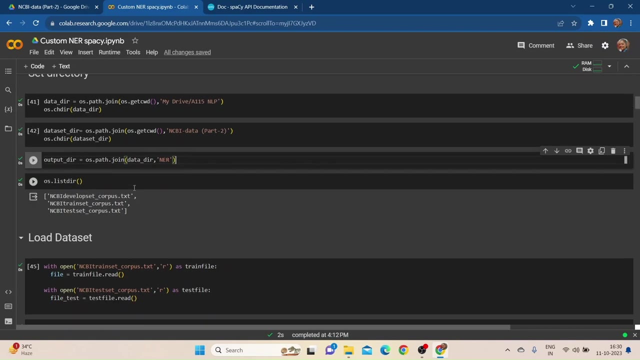 And then this is the dataset directory, where the dataset is present, our train and test set- And then we have an output directory where we will be storing the necessities for our model that we are going to use, Right? So currently we are pointing to this folder where we have our dataset. 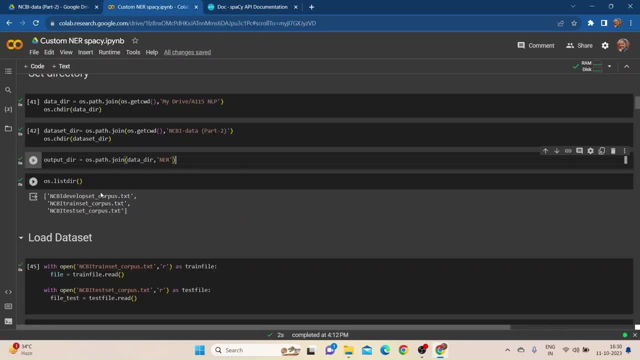 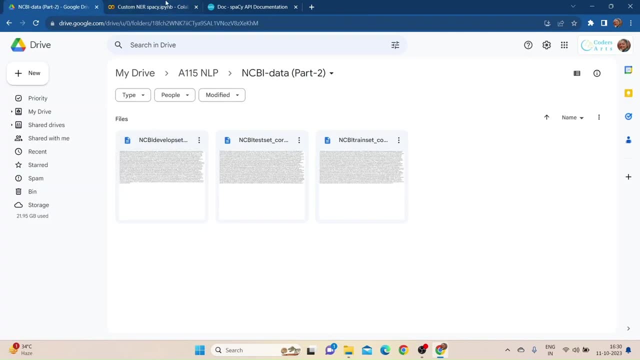 And here we are listing the name of the files which are present in the current directory And you can see that the train set corpus and test set corpus, along with the development set, has been listed here. We are not going to use the development set in this particular project. 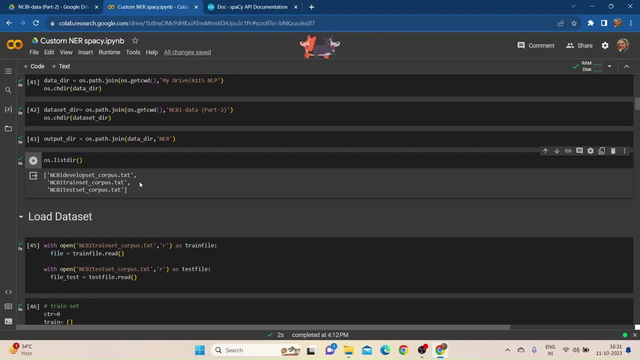 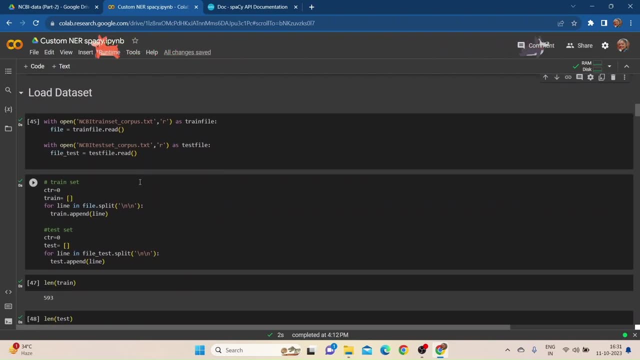 but it is a good practice to use development set also along with the train and test set. Okay, Now, after that, we do some pre-processing after loading the dataset. So the first step is to load the dataset And we are reading the text files here. 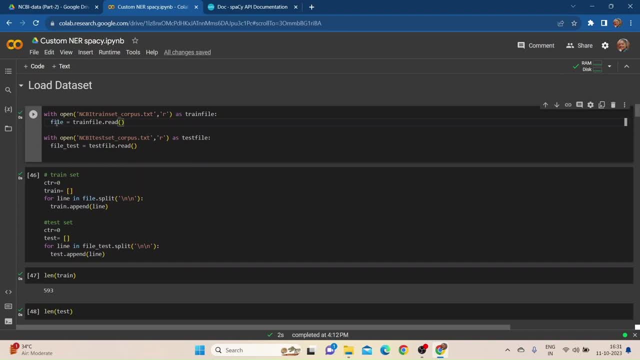 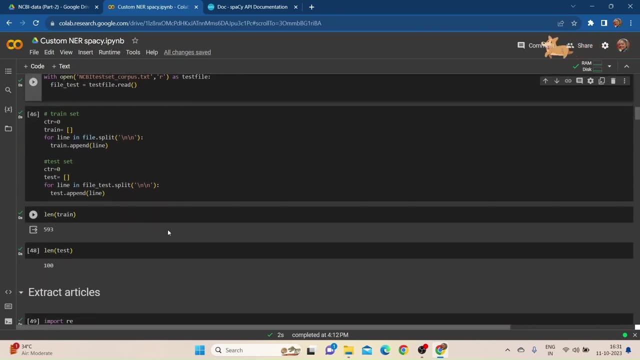 You can see that we are opening them in read mode And then we are just reading them and storing all the information from them in these variables, And then we are just creating a list for train and test data And the elements of these lists are going to be the different instances. 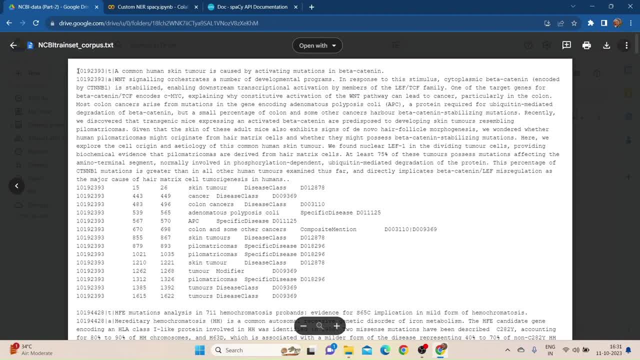 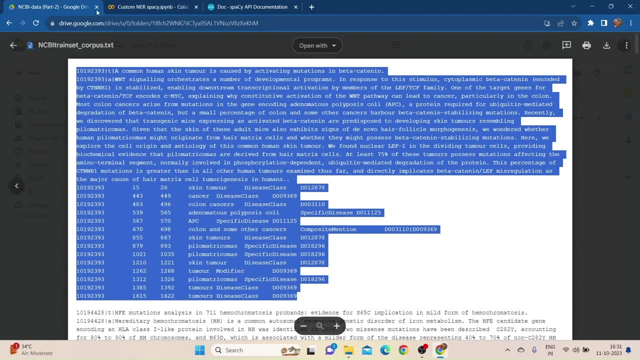 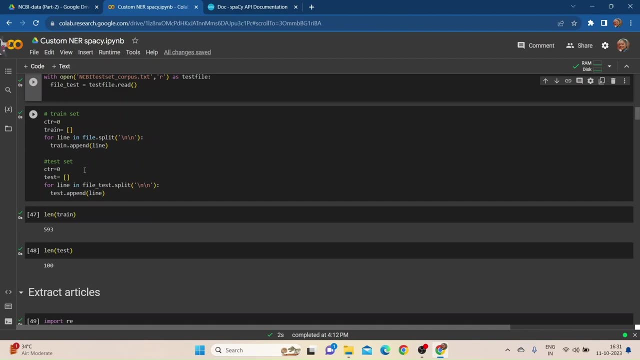 For example, here we saw that this particular data from here to here is one single instance. Okay, So all the instances that are present in the train data are going to be the elements of the train list, And similarly we are processing the test data as well. 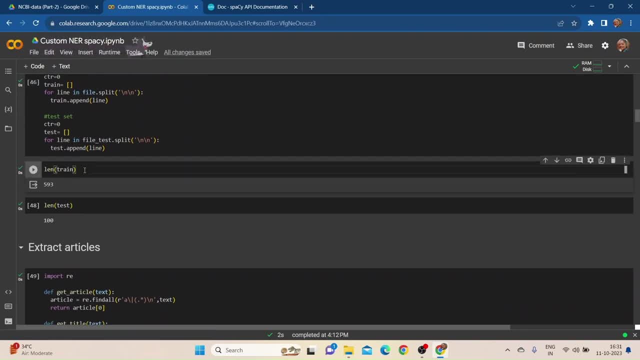 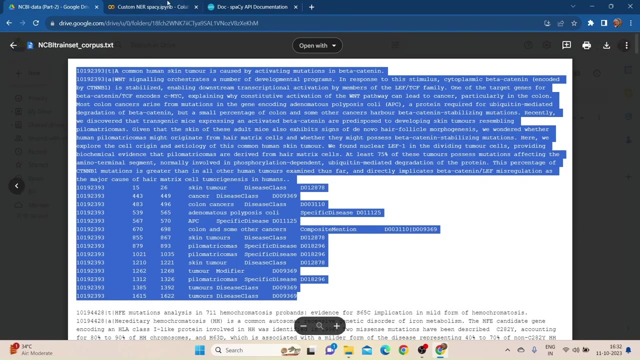 And on doing so, we find that there are 593 instances in the train data and 100 instances in the test data. Right After that, when we have extracted and stored this entire data in these lists, The next step is to extract the text separately and the annotation separately. 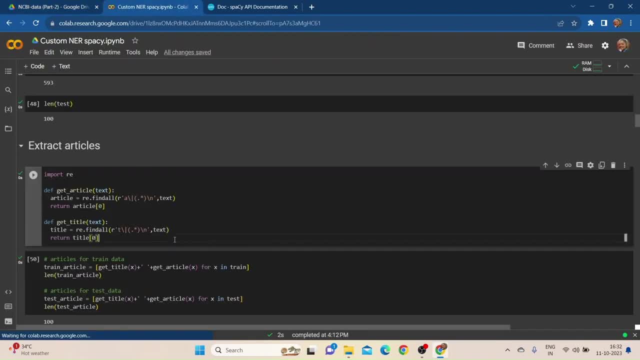 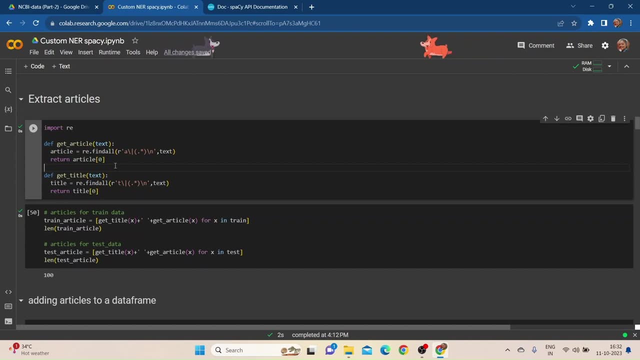 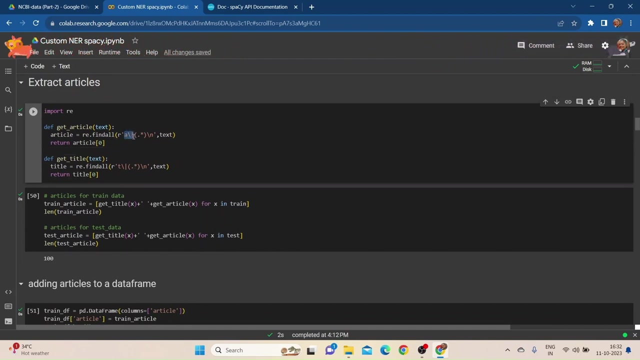 Okay, So first of all, here we have defined two functions, which is get article and get title, And in here we are making use of regular expressions to extract the particular data For the title and the body of the medical text. Right, The logic that we are following is that when the letter A is being followed by the pipe sign, 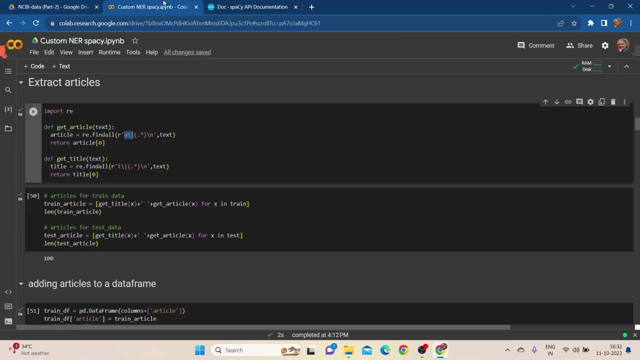 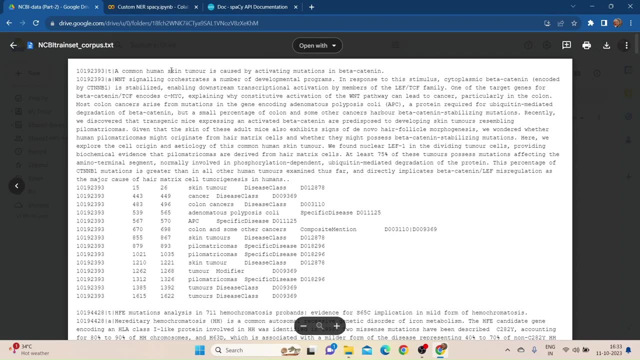 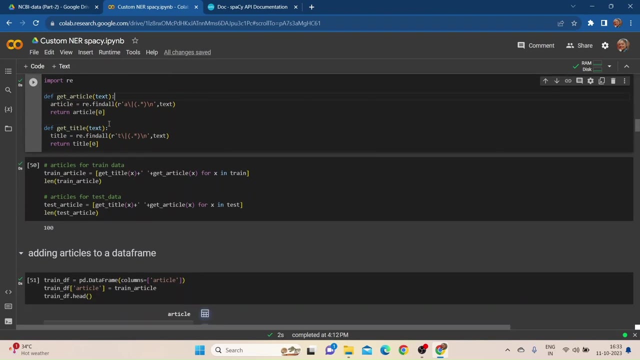 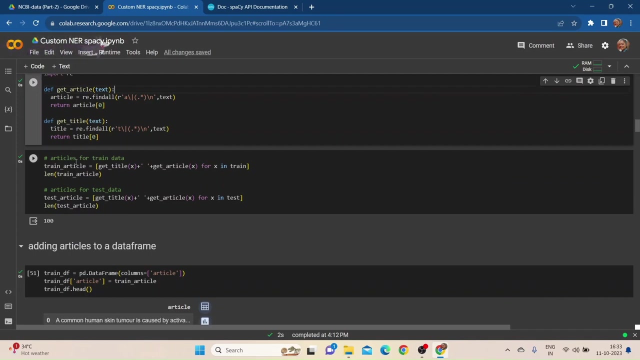 The text that follows is the article text. And similarly, when the letter T is being followed by the pipe sign, Then the text that follows is the title text. Okay, So we make use of these two functions to extract the relevant text And we are storing the article in another list called train article and test articles. 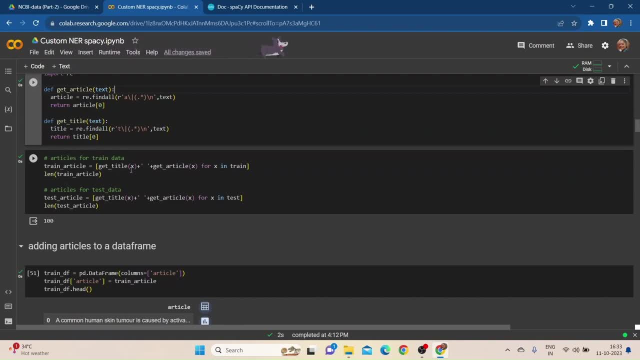 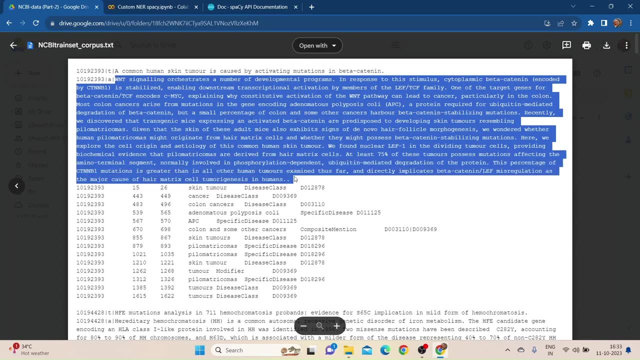 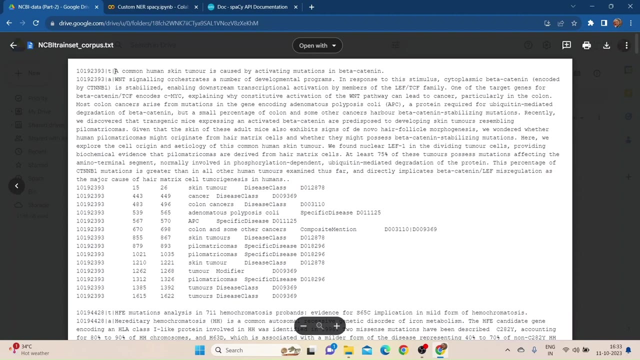 And basically, what we are doing here is we are concatenating the title and the article, Because I told you that the text of interest is not just the article like the body. We have to consider the title as well. That comprises of the total text that we are interested in. 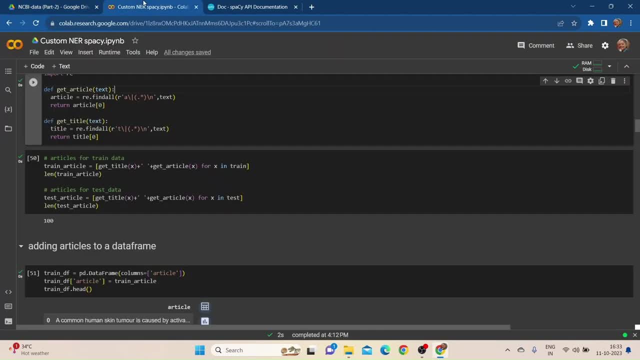 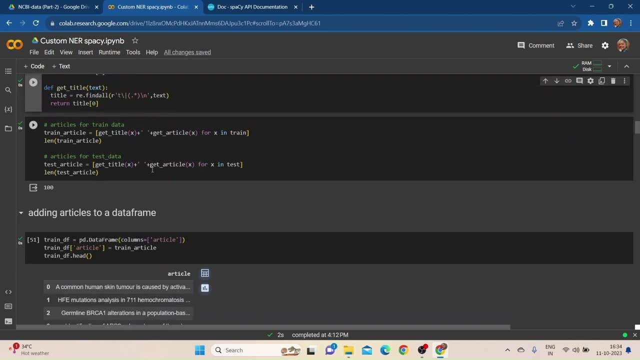 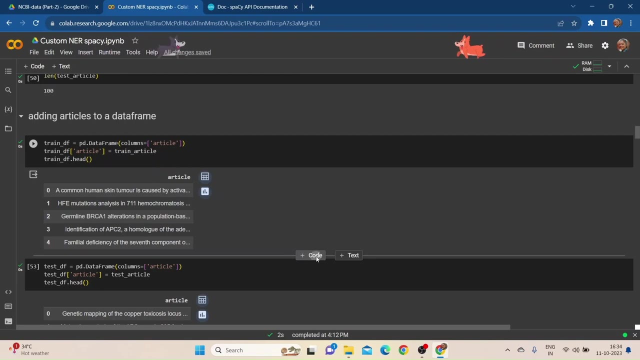 Because the indexing starts from the title, As we can see in the annotation. So here we are concatenating the title and the article And storing it into a list called article, And then we are just creating a data frame for better visualization. So you can see here the different articles that we have. 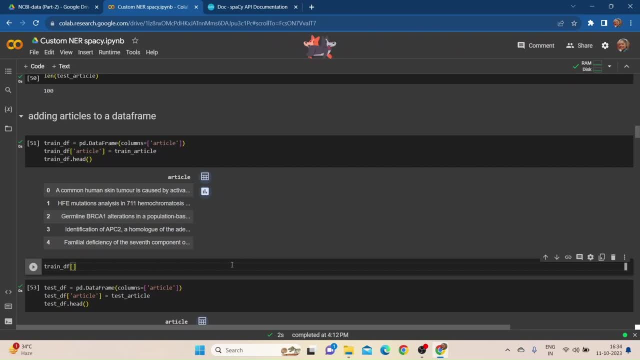 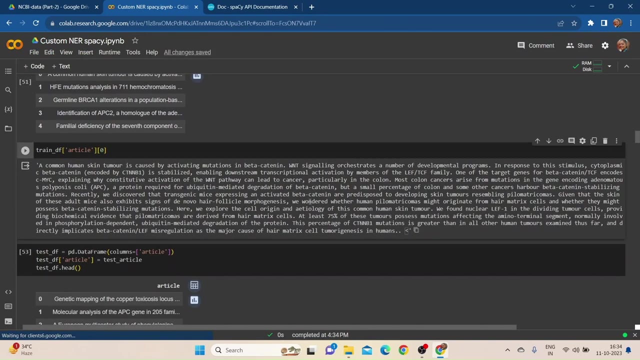 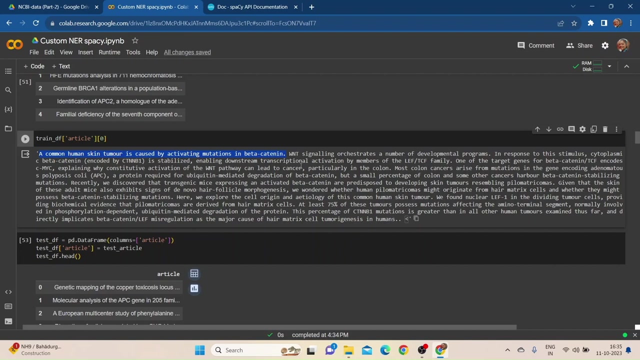 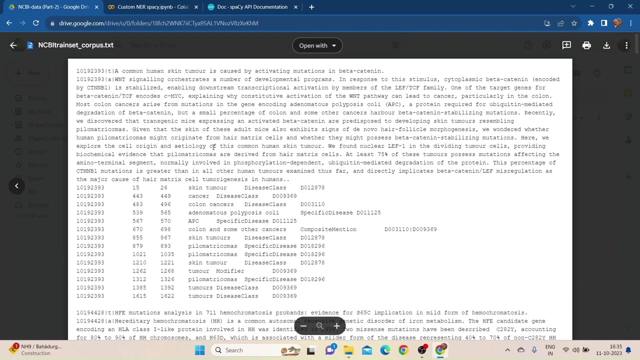 Let us just take a look at the first one. So here you see that this is the article. So in here the first line belongs to the title And the rest of the text belongs to the body of the medical text, And you can verify it from your training data. 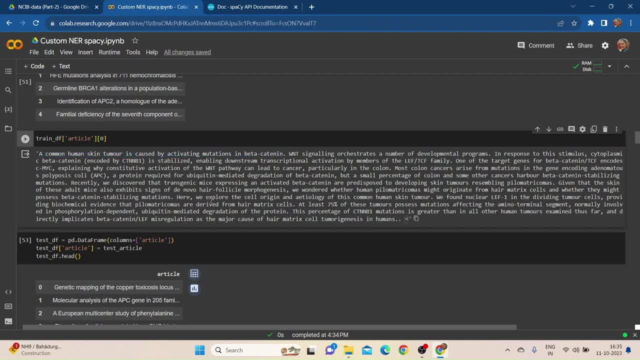 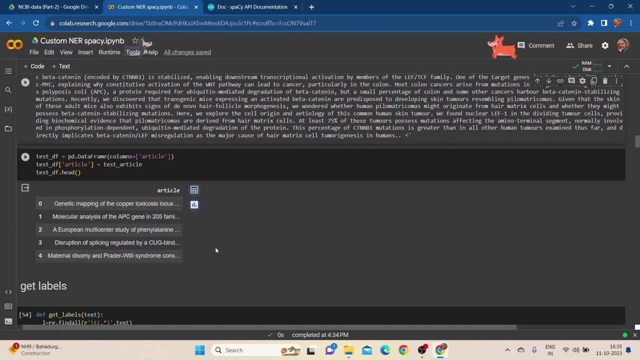 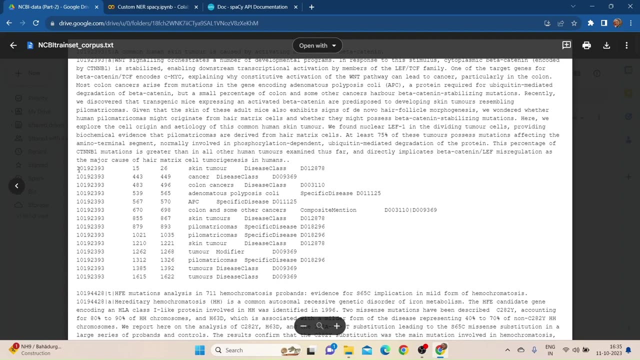 Just to check that the function is working correctly. Okay, And the same thing we are doing with the test data as well. Okay, Then, after extracting the text, The next thing that we need to do is to get the labels for the annotations. 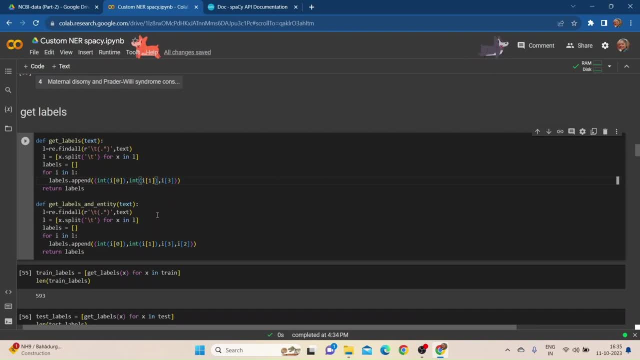 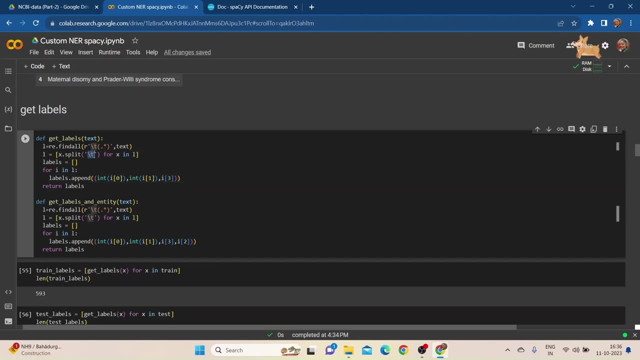 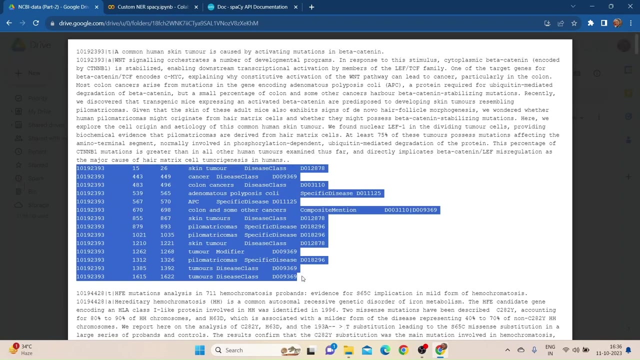 Okay, So for that also we have defined a function called get labels and entities, And the logic that we are following here is that the text are tab separated. Okay, So all the text that is tab separated Before the next line Is going to be considered as the annotation. 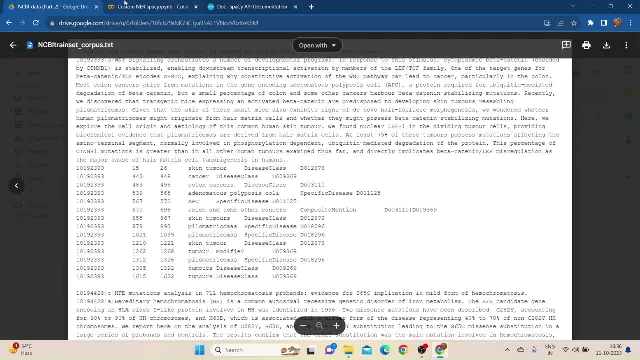 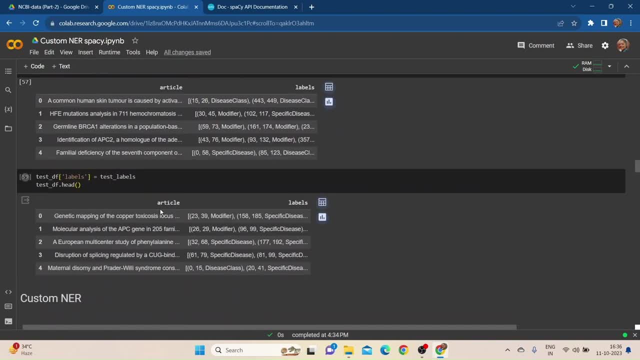 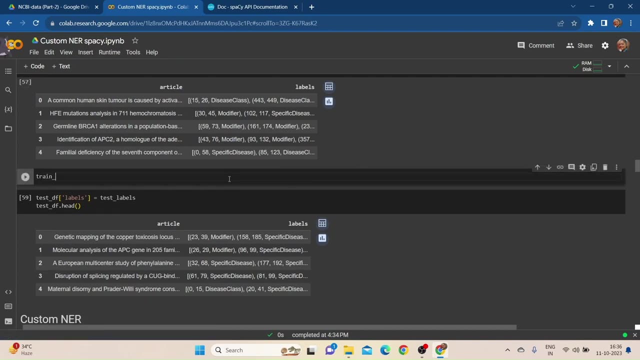 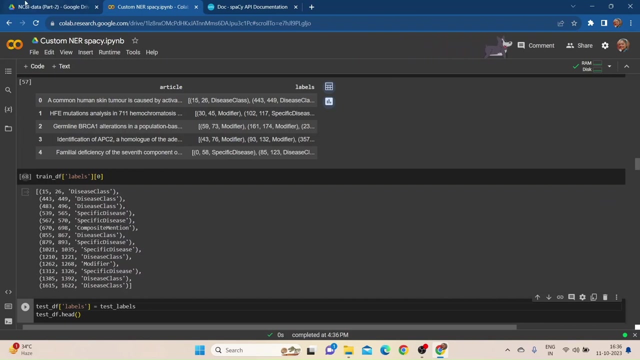 And even from this annotation, We are only extracting few relevant instances here, Which I will show it to you here. We have added this to the data frame as well. So just let us take a look what we have extracted. So you see that we have only extracted three things from this annotation. 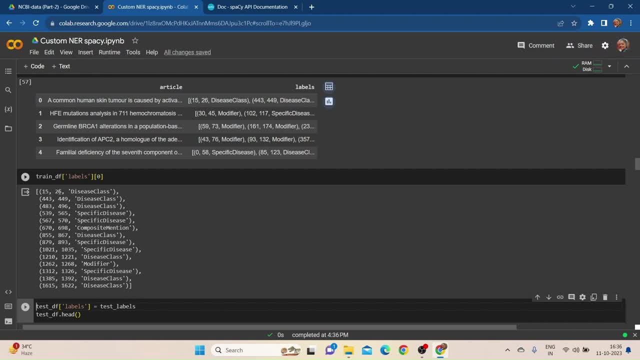 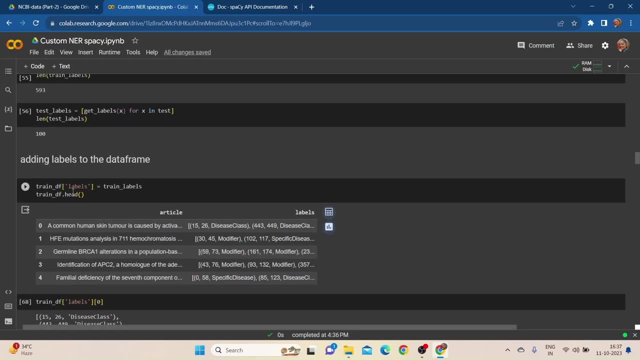 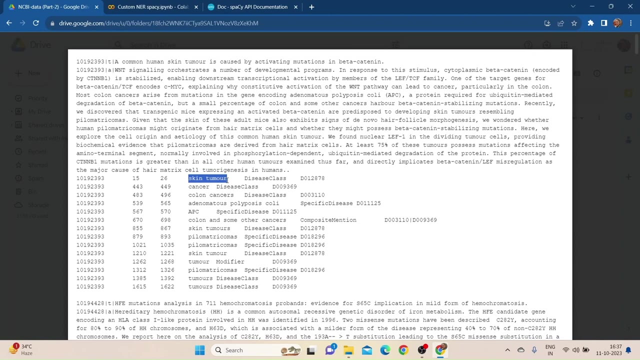 That is the start position, The end position of the word And the name of the category or the entity to which it belongs. Okay, So here. why we are doing so is because this data is basically redundant in nature. Right, Because we already have the text and we have the position. 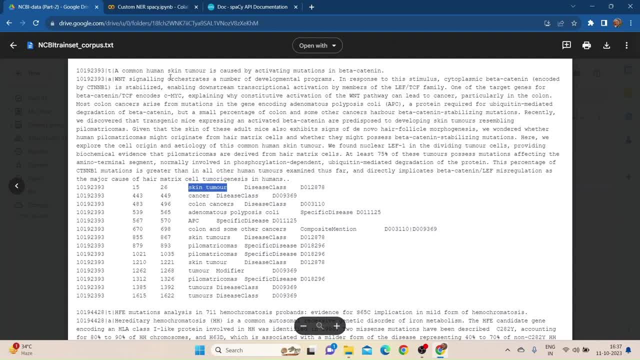 We can just, you know, find the word when it is required, Based on its position only, So we don't really need to extract this- And also from the category name and code. It's fine, It's sufficient to extract only one of these. 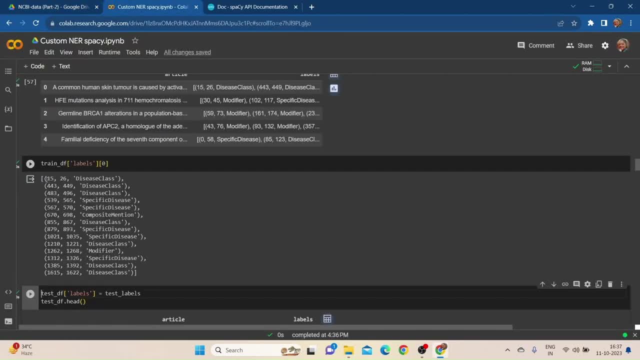 Okay, So this is how the labels are to be extracted And also, please note, the format in which they are extracted. This is a list of tuples, And each of the tuples is having three labels. Each of the tuples is having three elements. 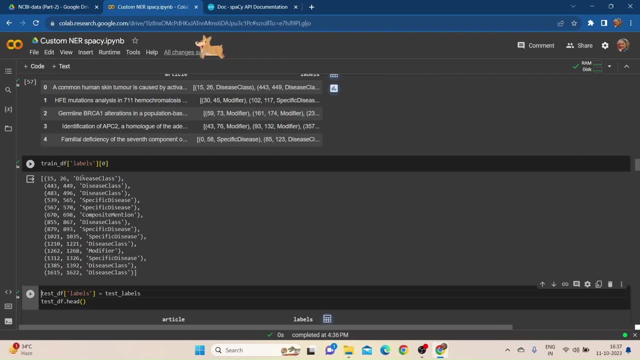 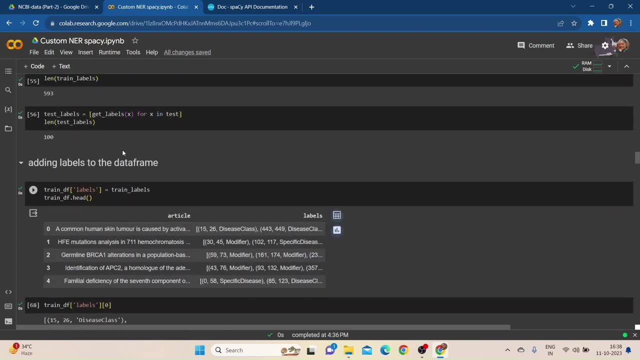 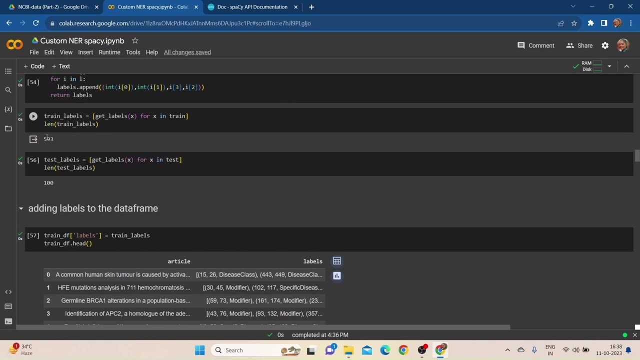 That is the start index, the end index of the word and the category to which it belongs to. So this format is very crucial and I will explain to you why. Also, please note that the instances in the train label is also 593, corresponding to the 593 articles that we have extracted. 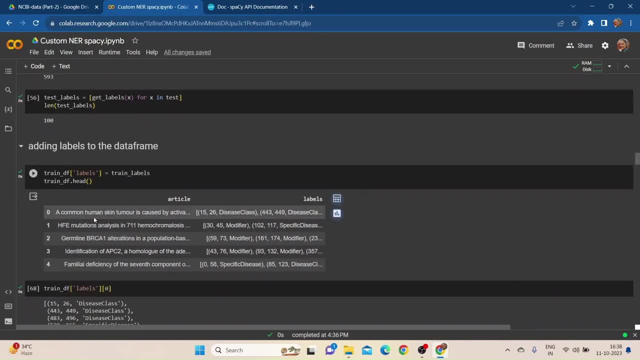 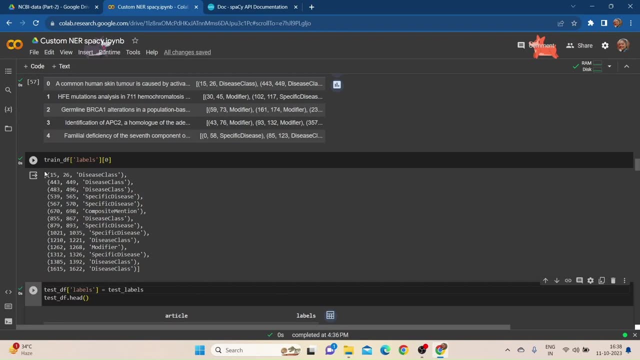 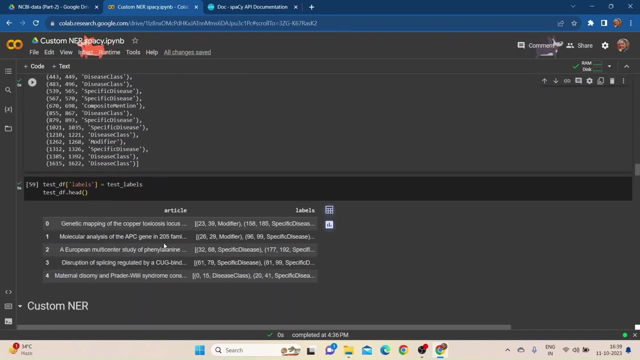 So it ensures that we have extracted all the annotations for all the articles. Okay, And in a prescribed manner as well, which is a list of tuples. So far here we have extracted the article and labels from the text files. Right Now we need to prepare the data for the model. 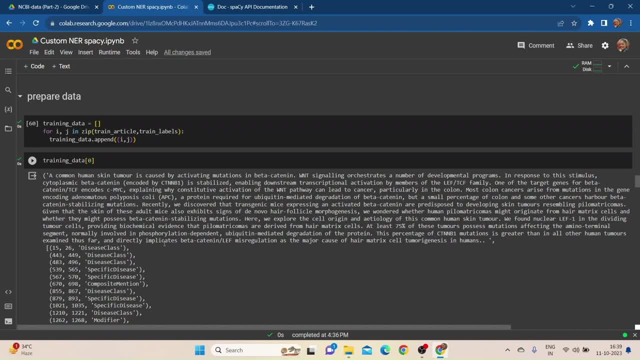 Okay For the NER model that we are to train Now. the model expects the data to be in spaces binary format And to convert the data into that format, We need to make use of spaces binary format. Okay, So in this case, is a docbin function? 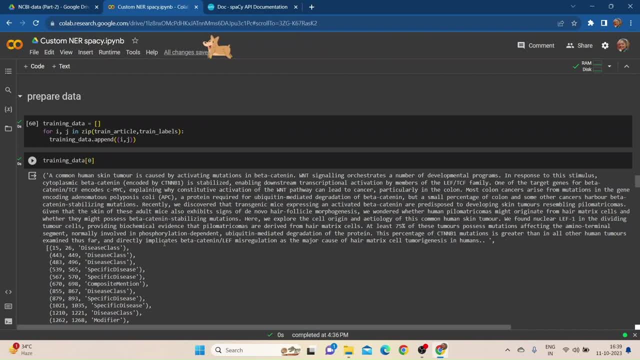 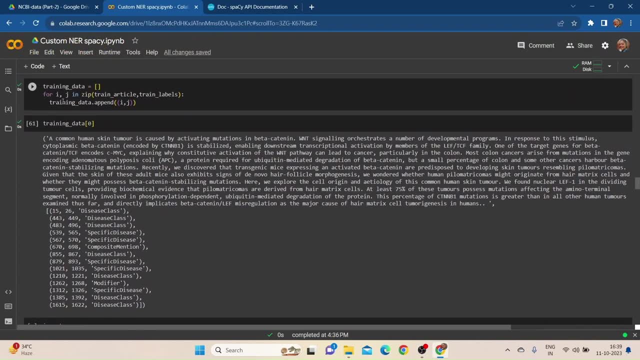 And that function requires the data to be into a specific format, which is this: Okay, So here we are creating another list which is basically called training data here, Right, And we can see the first instance in this list, which is entirely a tuple. 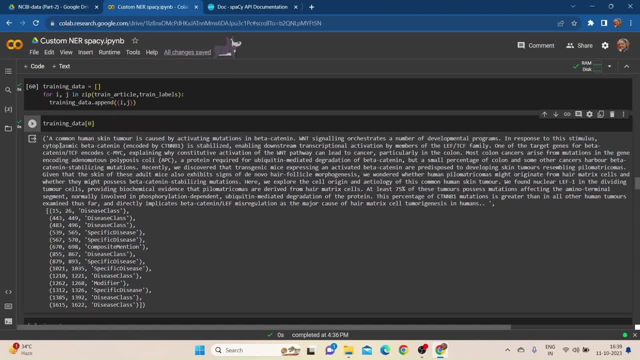 Okay, And this tuple is having two elements. The first element is the medical text itself. Okay, This text is, as we know, the concatenation of the title and the body, And then the second element is the annotation, which is a list of tuples. 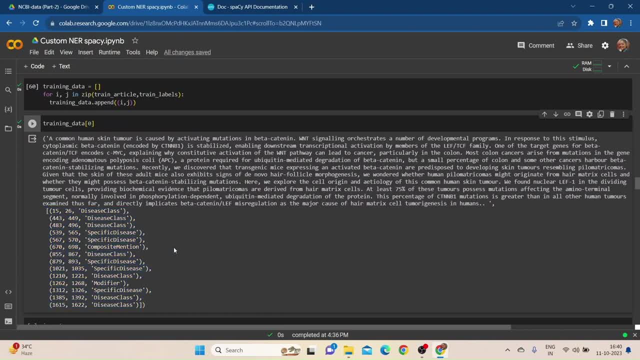 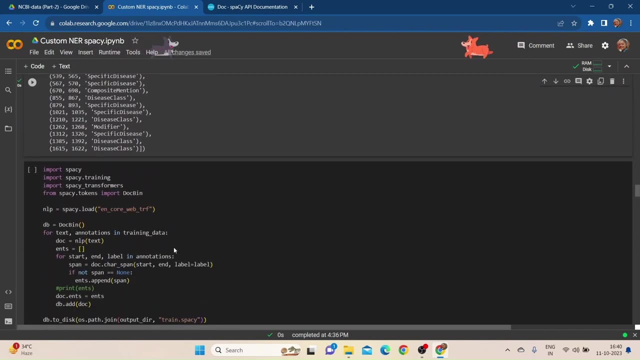 And each tuple is having three elements in it. So this is the expected format for the docbin. Okay, So that it can convert this data into spaces binary format which is supported by the model. Okay, So here we are making use of docbin to convert this data into the binary format. 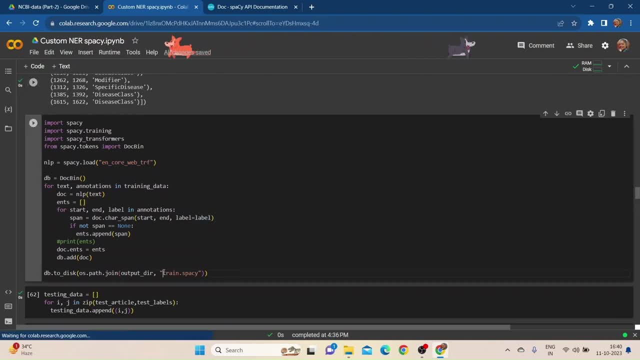 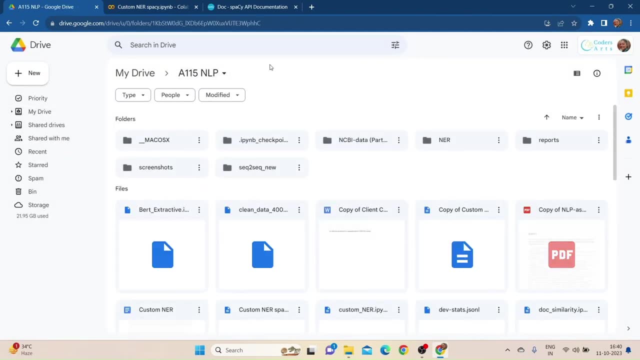 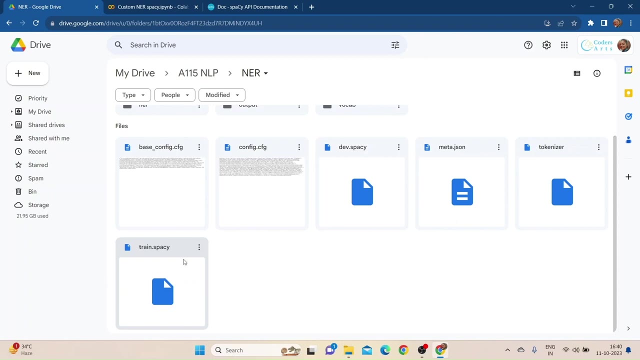 And it is being saved as trainspacy in the output directory. Let's just check if it is present there. So this is the output directory And we can see that we have trainspacy here, And even the devspacy is also there. 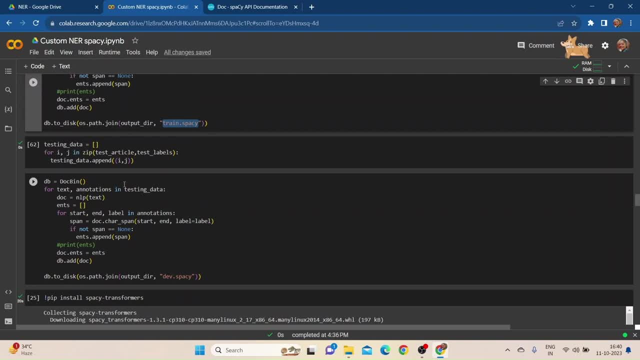 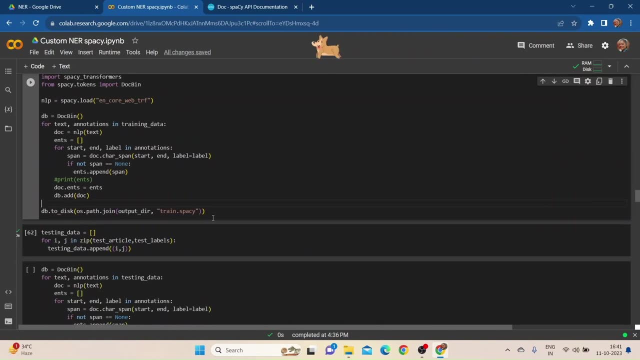 devspacy is the binary format for the testing data. Okay, So by this point here we have pre-processed our data And now it is into a format which is suitable for model And we can train the model using that format of the data. 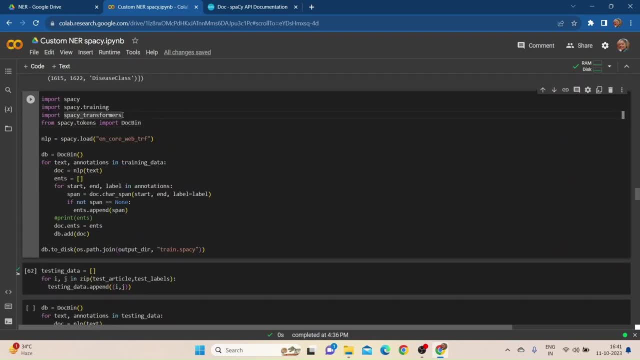 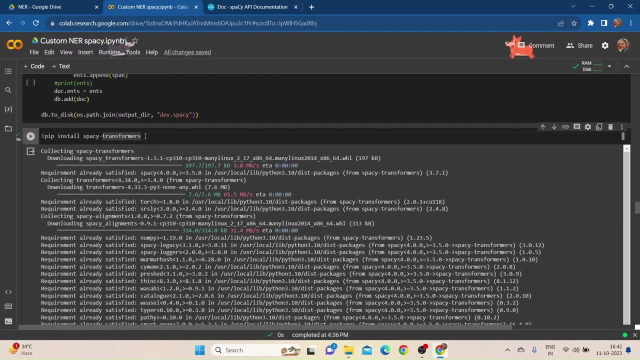 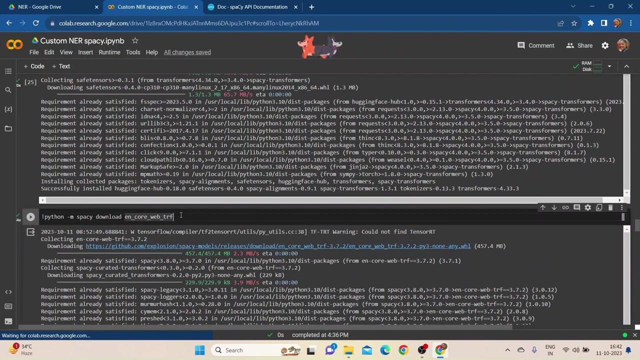 Now please pay attention here that I have imported spaces transformer And also I have loaded the English language space model With transformer support. Okay, So for that you will need to first install the spaces transformer like this, And you will also need to download the English language model, which is having the transformer support by following this line of code: 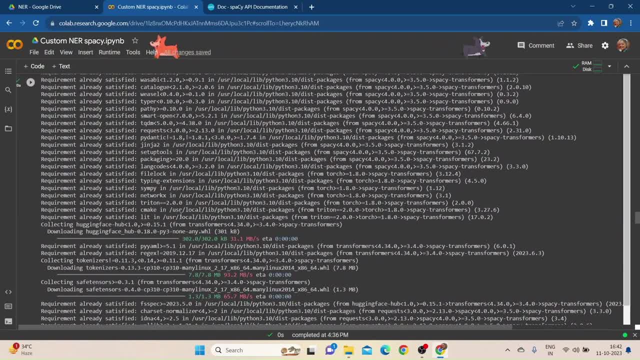 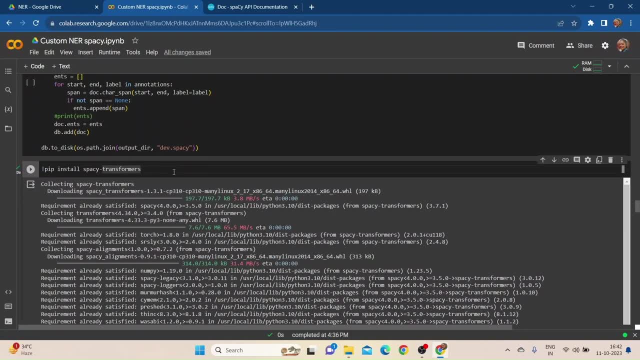 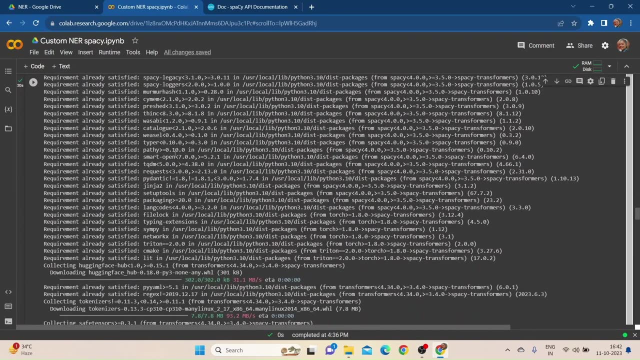 And please don't mind that I have done it later. At the time of development I forgot to do it And when I encountered the errors, I installed it into the subsequent cells And it remains so. So please ignore, Right, But it is necessary. 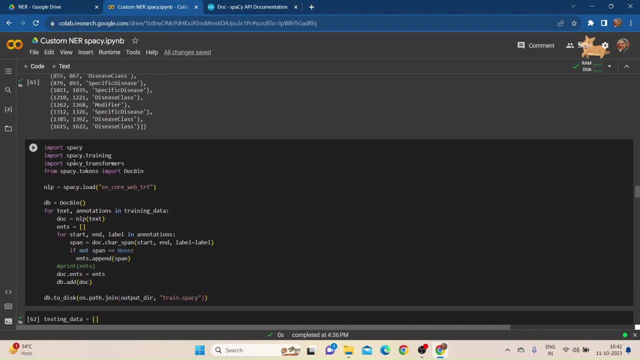 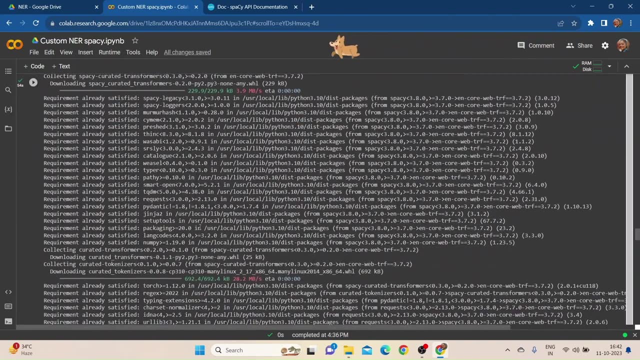 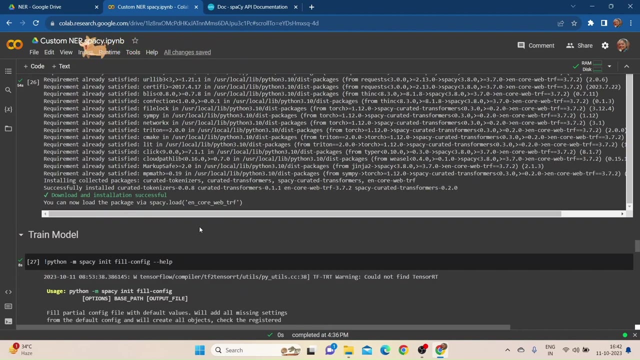 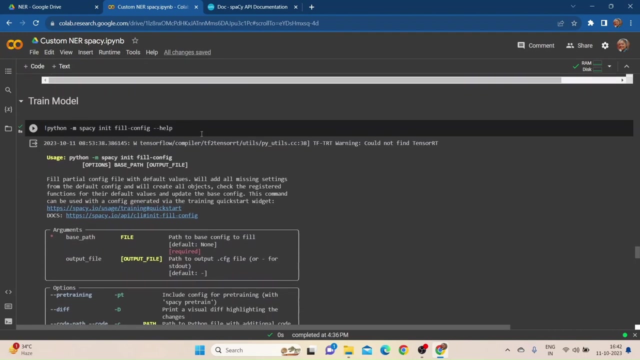 And I suggest that you do it before importing these libraries. Then here we come to the training part. Now the data has been pre-processed And it has been converted into the binary format, So we are ready for training the model, And here, in this line of code, we are doing nothing. 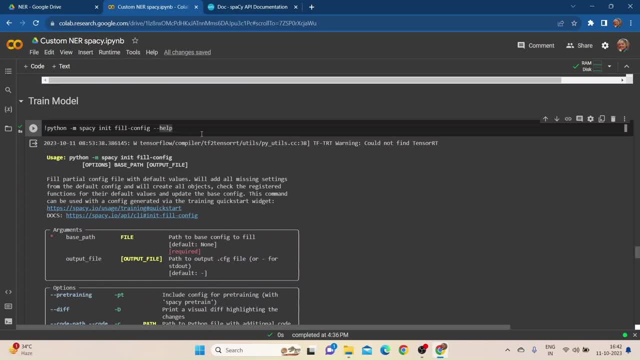 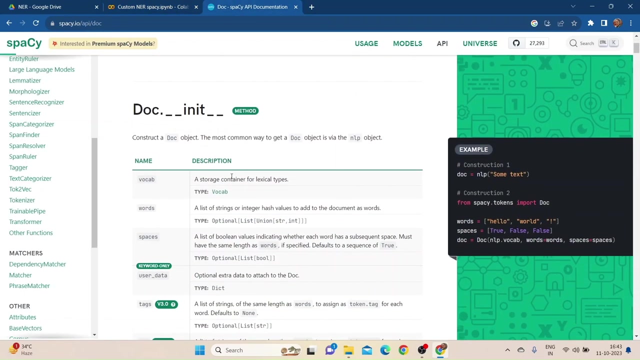 We are just, you know, printing the help to generate the configuration file. Okay, And here it is specifying the usage or basically the command which is to be followed to generate the configuration files for the NER model that is to be trained, Right. So all this you know, commands you can find in the documentation page of spaces. 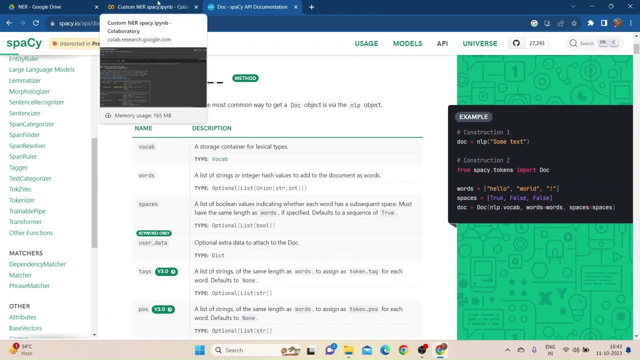 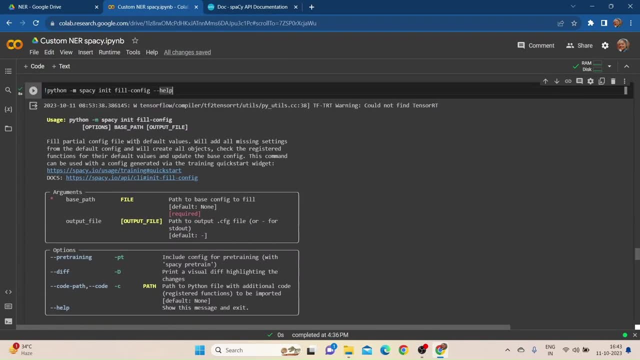 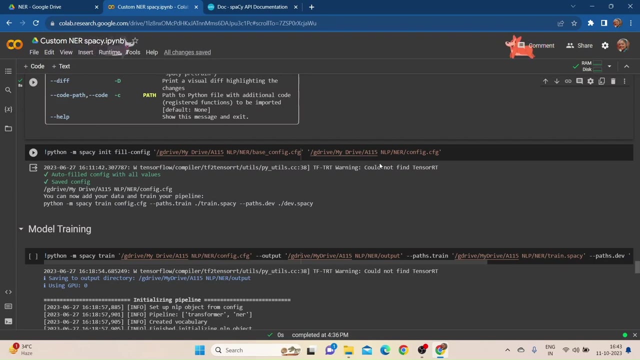 Okay, So that's why I encourage you to follow this documentation when you are working with spacey And based on this usage. here we are just downloading the base configuration and the configuration files for the model, And it is also going to be stored in the output folder here. 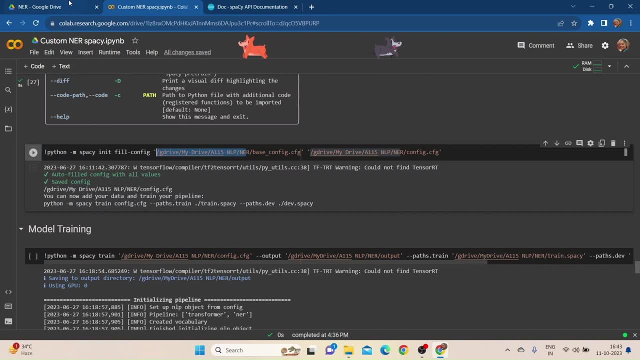 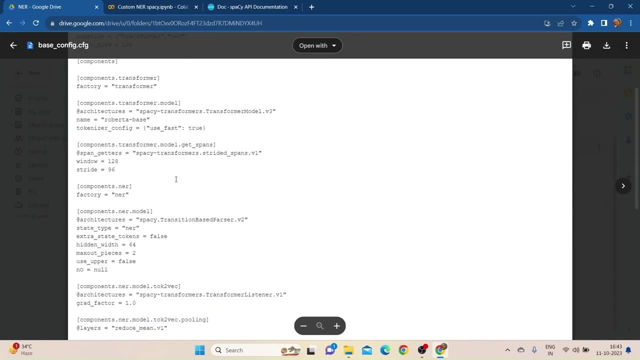 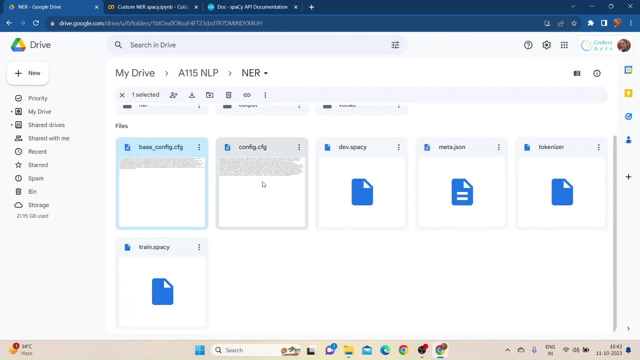 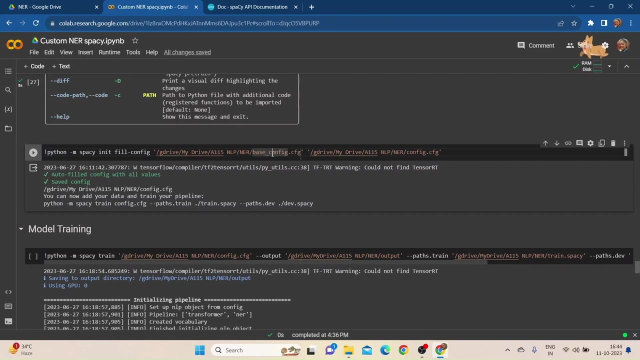 We are given the path accordingly And you can see here this is the base configuration file, Okay, And it is having some parameters which are having some values. These values are going to be used by the model at the time of training. So installing or downloading the base configuration file is very necessary so that you are able to train the model. 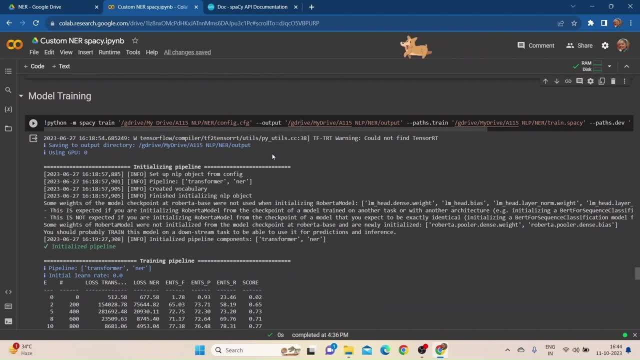 And after that comes the most important part, that is, the model training. Now just let us take a look at the code. Here we are running a command where we are instructing spacey to train the model with the configuration, And here we are passing the path to the configuration. 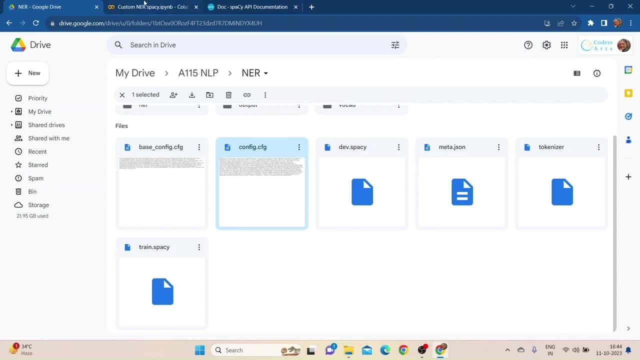 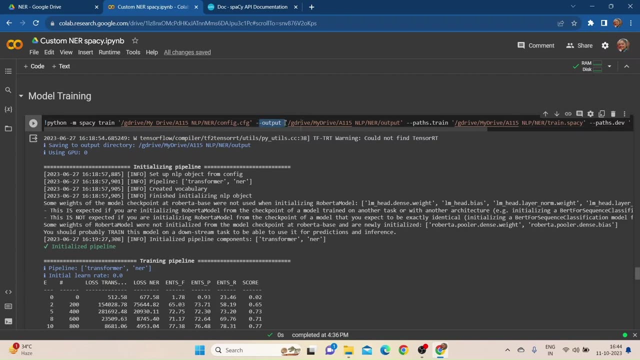 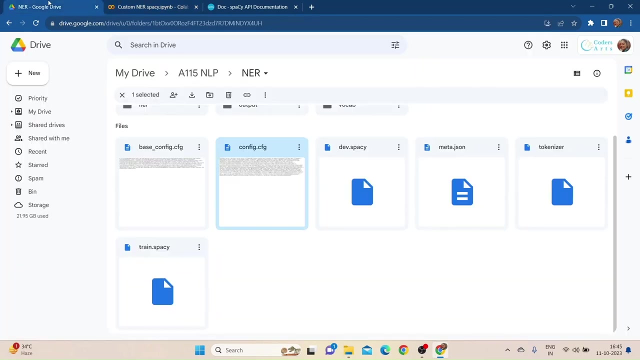 Okay, So we are basically pointing to this configuration file, which the model will be using at the time of training, And the output is to be stored in the output folder. Okay, And the output basically is the trained model, And then we give the paths to the train and development binary files that we have generated. 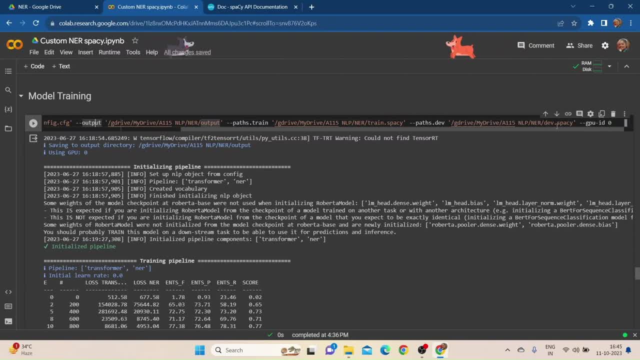 Basically trainspacey and devspacey, as you can see, And here we are giving the id of the GPU that is to be used- I highly recommend that you use GPU at the time of training, because it is a time taking process And it will take quite a while to train your model. 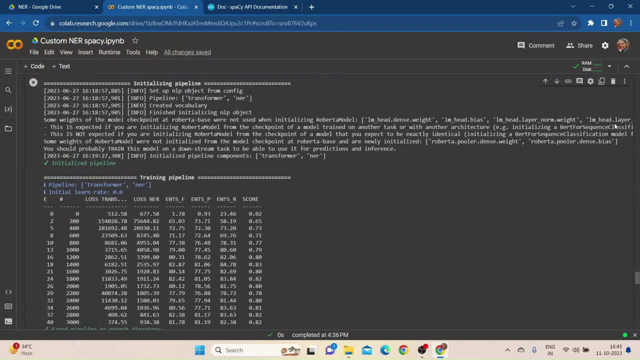 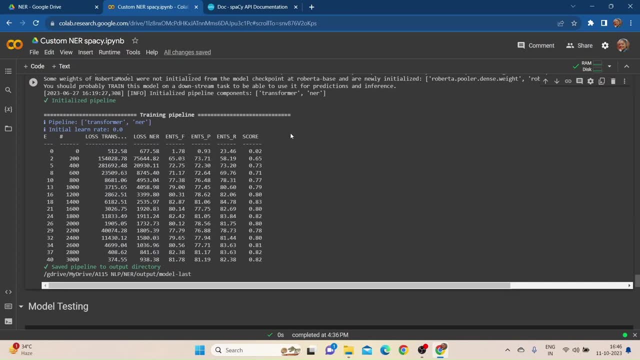 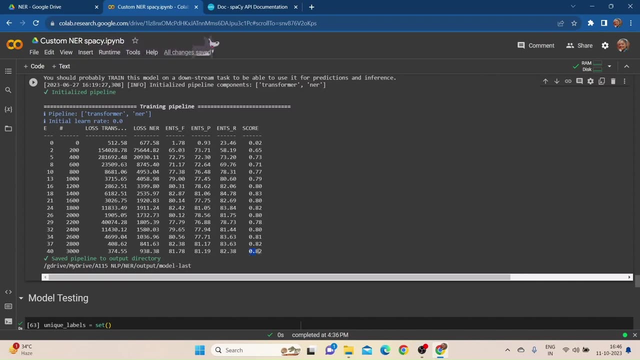 So, in order to speeden up the process of training, I suggest that you use GPU. Okay, So here is the results of the training. We can see that we achieved a score of 82%, And it is pretty good, I would say, because in NLP, achieving higher accuracy is very difficult. 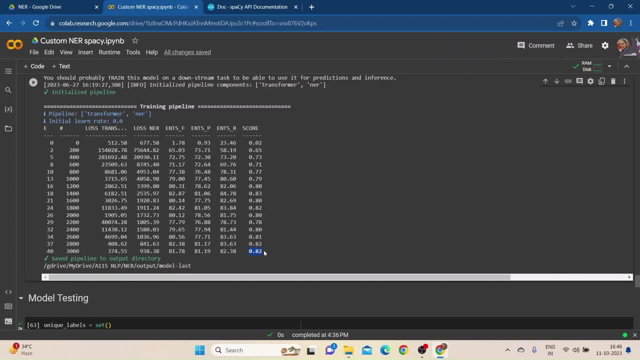 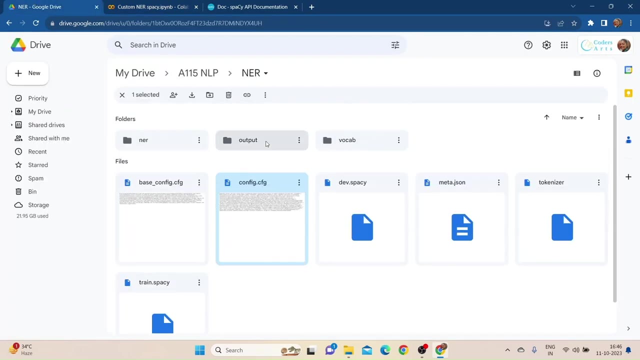 So this is also a decent score. You can see that at the time of training it prints the loss of the NER model along with the F1 score, precision score and the recall score, And the model is saved here in the output folder as it has been instructed. 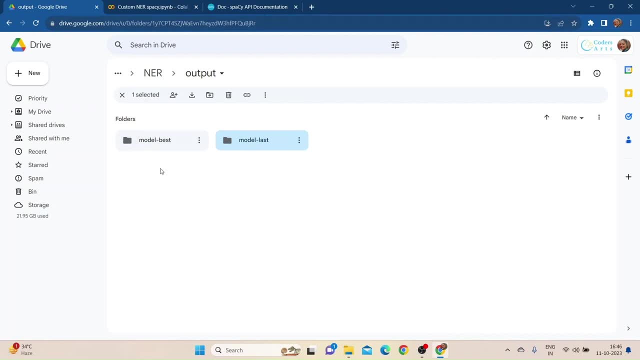 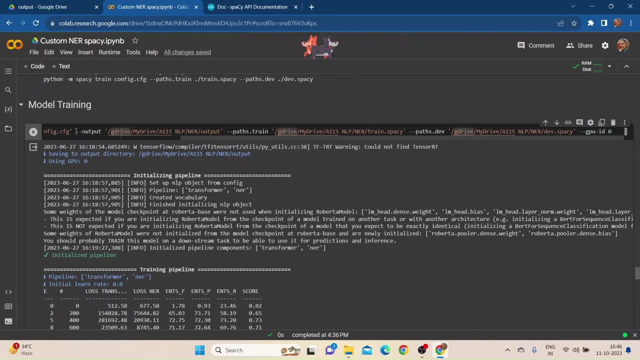 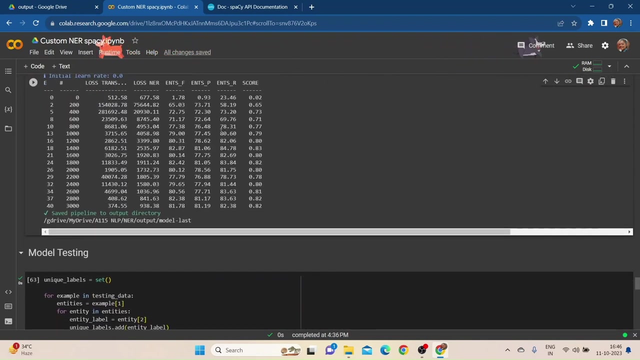 Right, So we see that the last model and the best models are stored in this folder Here. we instructed it to save. Okay, So we can see that the last model and the best models are stored in this folder. Okay, Now that we have trained our model, we can test it. 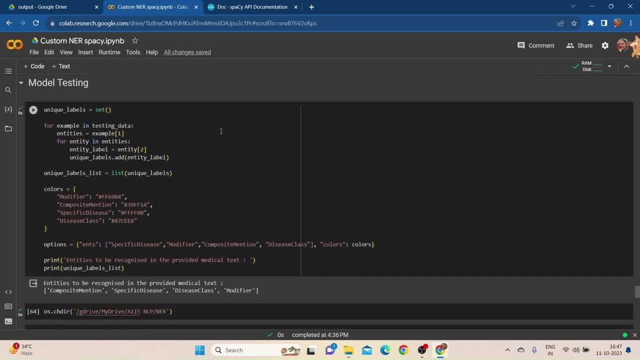 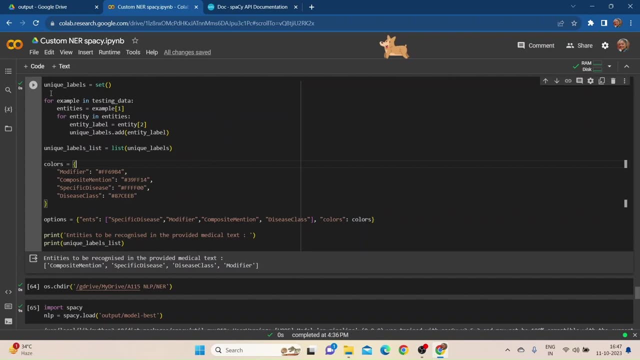 So we come to the testing part, And in order to display our code in a beautiful manner, we have written some code for that as well here. So basically, in this cell, what is happening is we are just getting the unique labels from the annotation of the data. 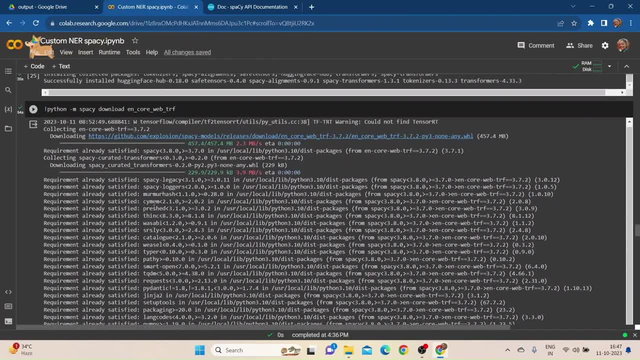 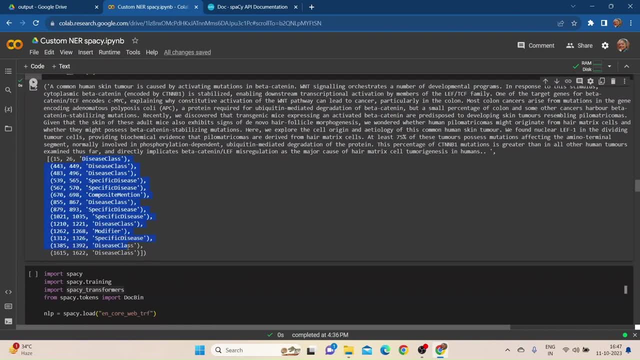 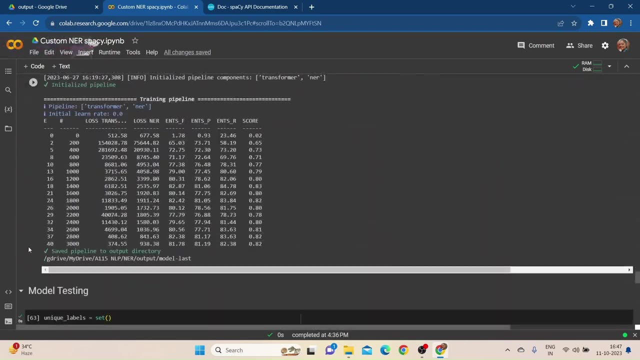 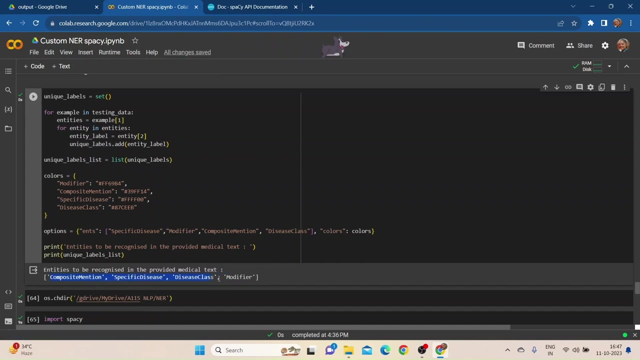 Okay, So basically from this part, Yeah, So we are analyzing all the annotations And from there we are just getting all the unique categories or entities which are present in the data set that is available to us, And we find that there are four unique entities. 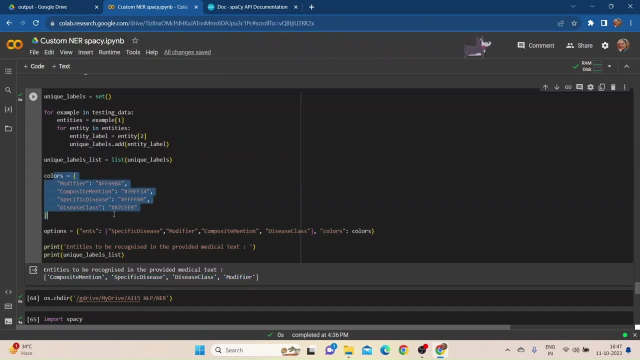 And then we are, you know, specifying a color scheme for each of these entities here in a dictionary, And then we create another dictionary of options where the entities are listed, And also we are giving the color scheme for each of the entities, And then we go to the directory where the model output has been stored. 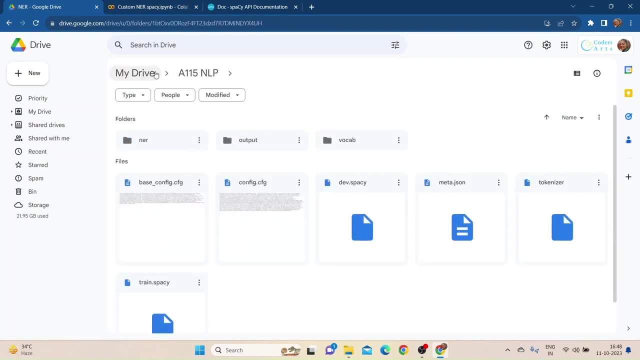 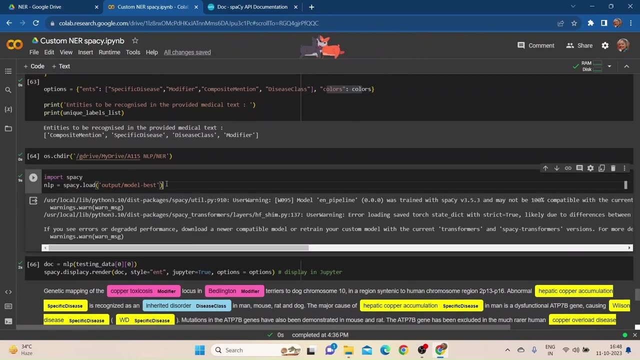 Okay. So basically, what we are doing is we are coming to this particular directory And then we are loading the best model. Okay, So we are not using the last model, but the best one. We load it And store it into a variable called NLP. 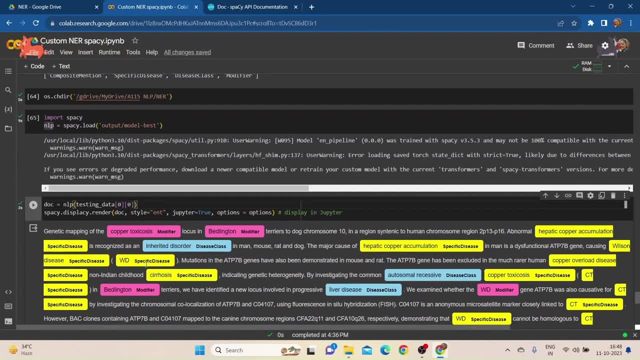 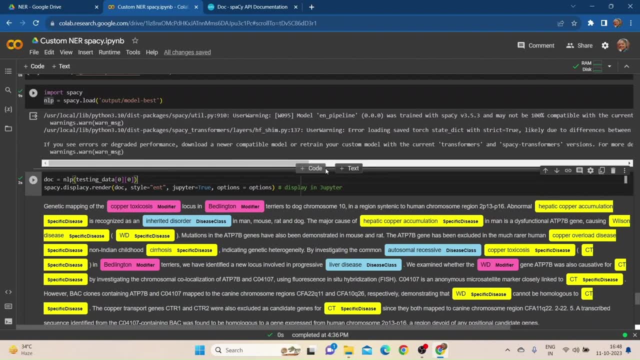 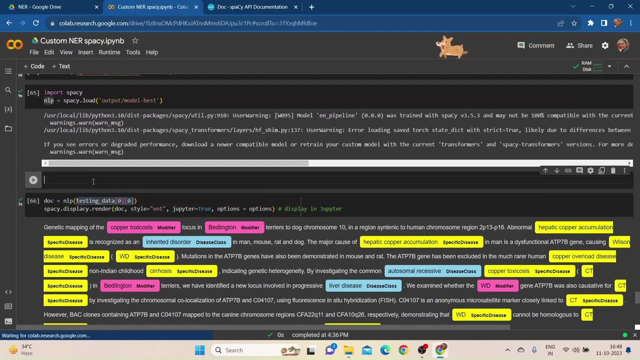 And here you can see that to this model we are passing in the text part only of the testing data, The first instance of the testing data. Let me just quickly show to you as well what I mean by that, So you can see that this is the. 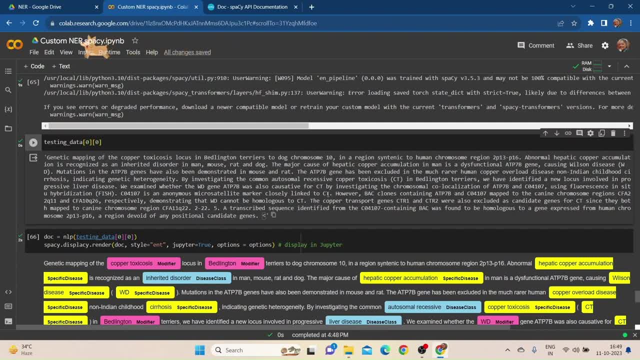 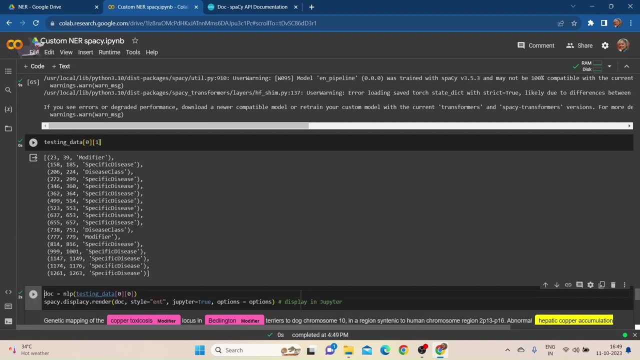 This is only the medical text, Not the annotation part. Okay, So this index 0 here represents the first element of the testing data, which is the text, And the second element, if you will see, is going to be the annotation. But we don't need to pass in the annotation at the time of testing. 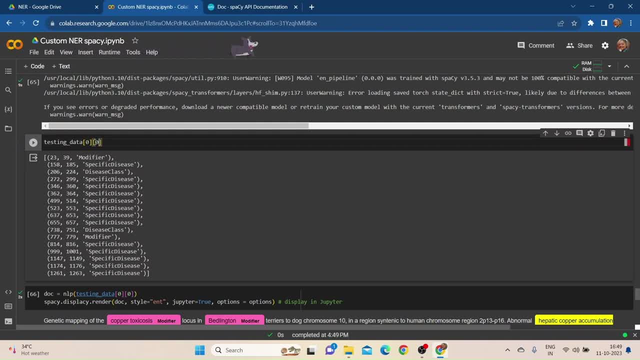 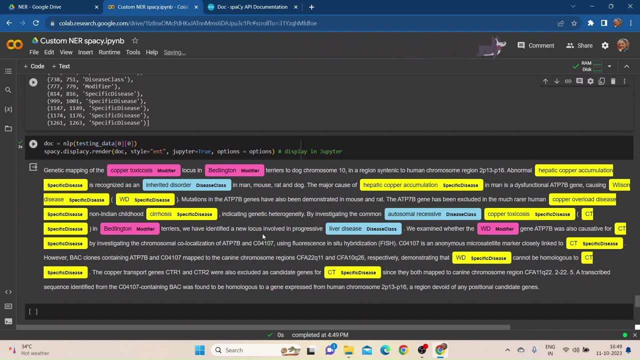 Okay, So let's just make it 0.. So this is the result here. You can see that different entities Are being recognized in the text, And to visualize this result in this beautiful manner, We are using spaces or displacy To render named entities in the provided medical text, along with the color scheme. 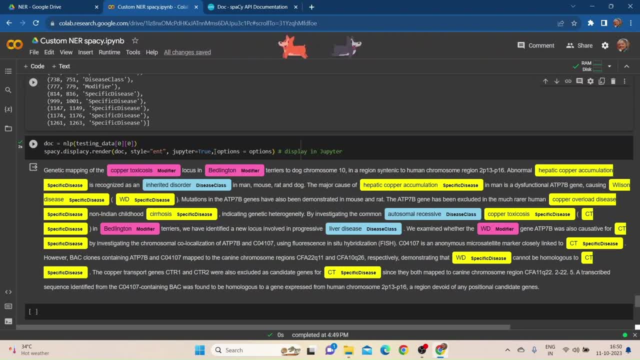 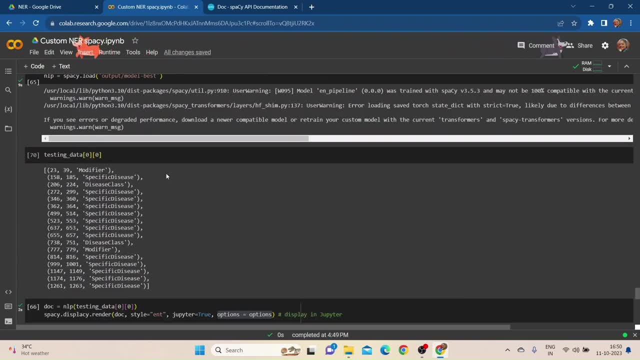 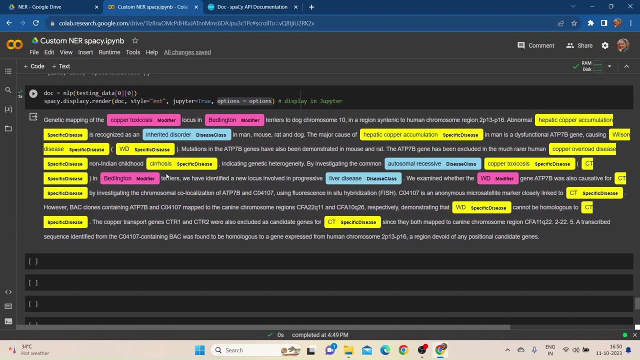 So you can see here that in displacy only, we have passed in the options dictionary that we created here, Where the color scheme for each of the categories is present. So this is the output And you can see that now the model has learned to identify the entities in the text. 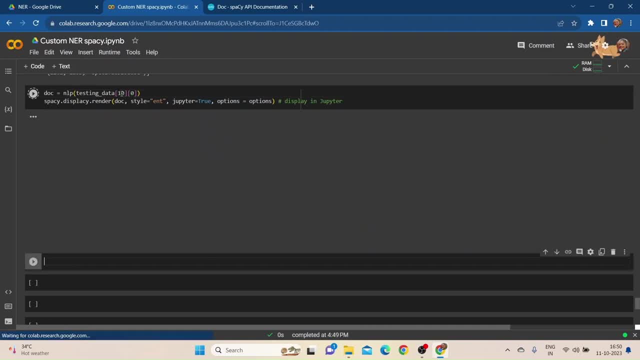 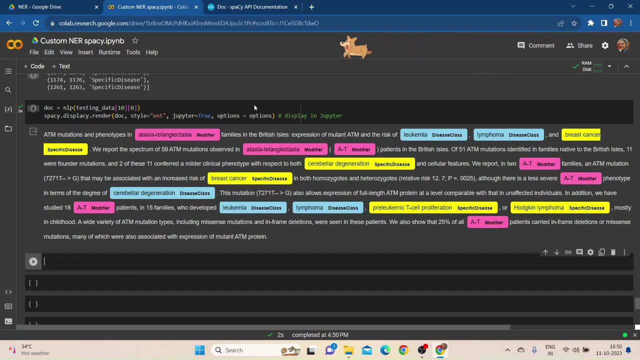 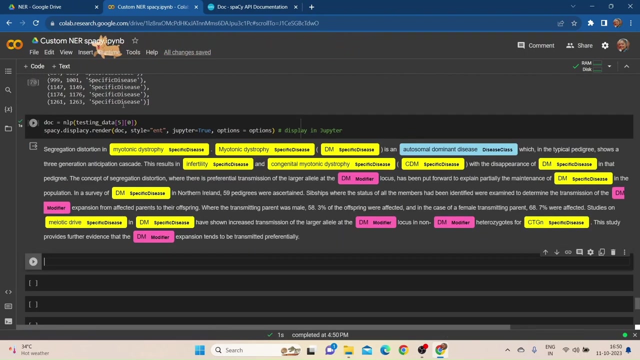 We can check it for different instances as well. Let's see, It takes nearly seconds to recognize the entities, Right? Let's just check another instance. So this is how we can use NLP and basically NER to extract or identify entities into medical text, or not just medical text, but any kind of text. 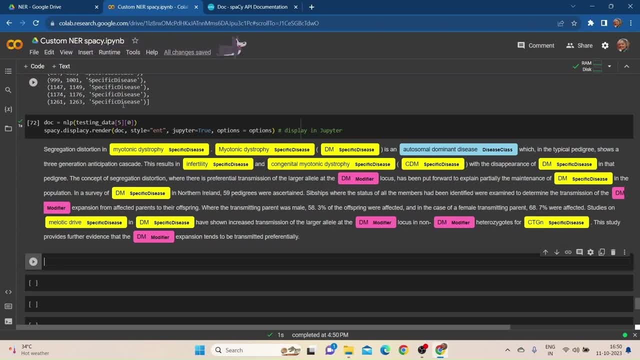 Given that we have the training data for it. So finally, let's touch on some challenges in NER. The first challenge is ambiguity, That is, some words can be classified differently based on context. We all know this. We all know that English is a very funny language. 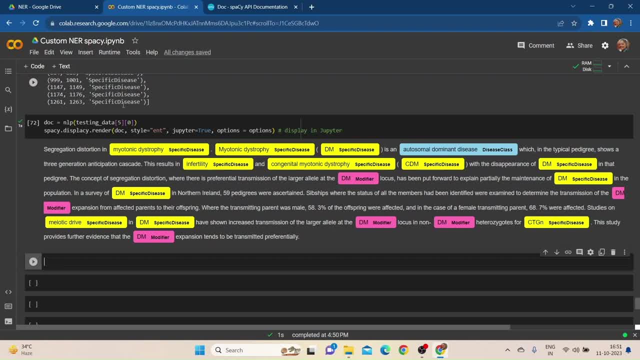 And one particular word can have several meanings based on its context, Right, But teaching this context part to the machines is really tricky And like the research is still going on in this department, Because currently in NLP identifying the context is very difficult. 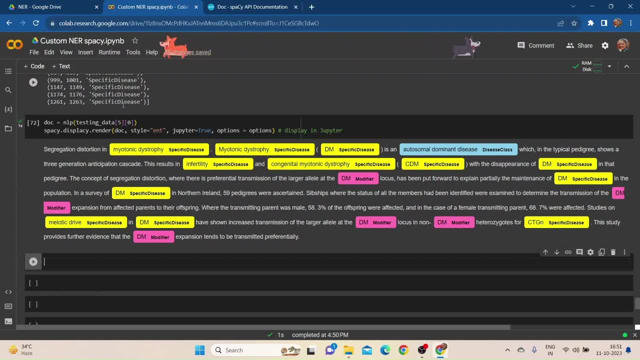 And there is no perfect implementation Of understanding the context so far. So this remains to be one of the major challenges in NLP, not just in NER. Then there is variation in the named entities as well, Because names can be spelled in various ways. 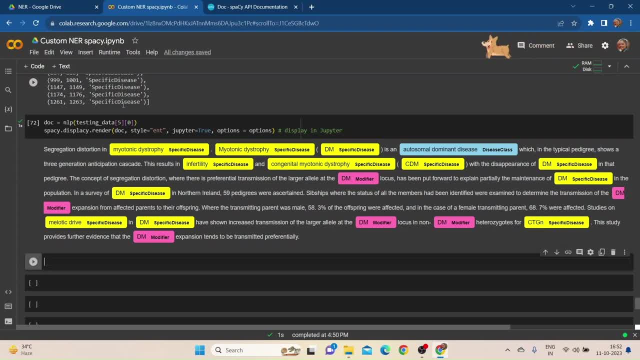 Right, We have seen that quite a lot of people have different kind of spellings for similar kind of names. And not just that. We can see that we have US version of English and then there is a British version of English And there is a slight change into the spellings of particular words. 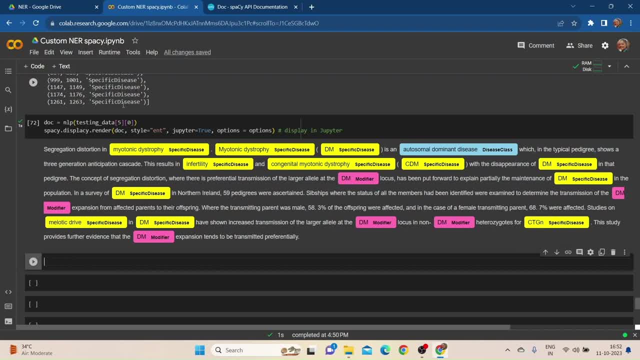 Right, So that also creates ambiguity for the model. Okay, So that introduces a challenge to the model. And then domain specificity also is a challenge. NER models may not work well in highly specialized domains without domain specific training data. So basically, in this case we had the medical data which was annotated. 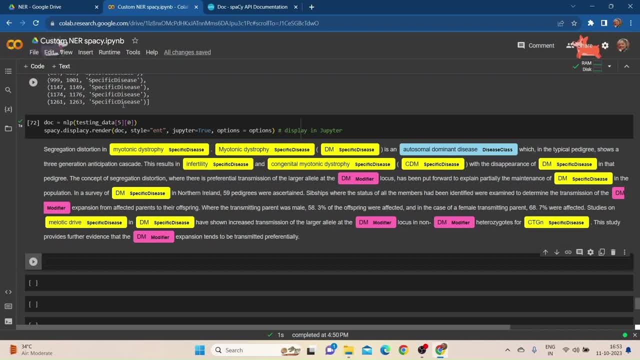 And that is why we were able to train such a model to identify the entities into medical text- Right, But if, let's say, we have to create a model for identifying entities in legal documents, Then we will need training data Relevant to that kind of documentation. 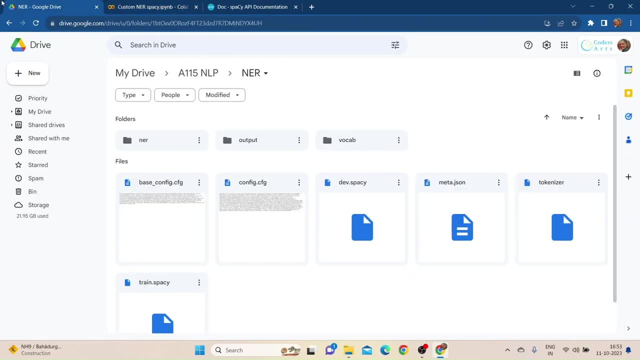 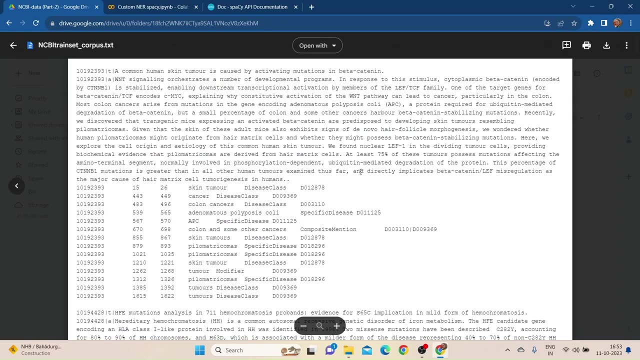 Right? So this kind of data that we are using here is not going to be suitable for creating a model that is going to recognize the entities into legal documents Or, for that matter, in construction documents. Right, So for each specific use case in various industries. 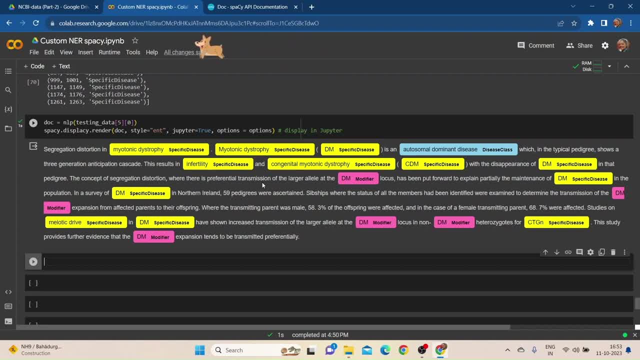 We will need training data And not just training data, Annotated training data, Okay, And it is a time taking process, So this also is a challenge in developing such kind of models. Right, But if we have enough data for training, 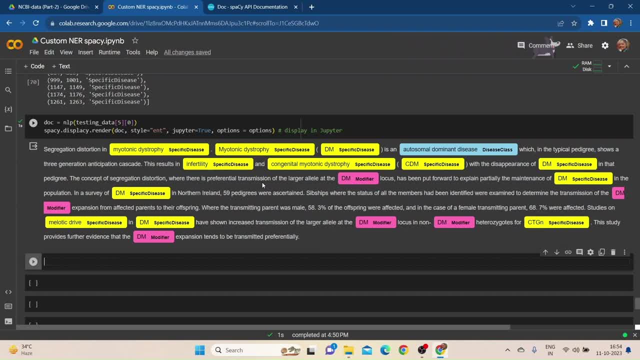 If we can create annotated data, Then we can surely implement these kind of models for different kind of use cases. Okay, So in conclusion, I would like to say that NER is a vital tool in the field of natural language processing, Which is helping us to extract valuable information from text data. 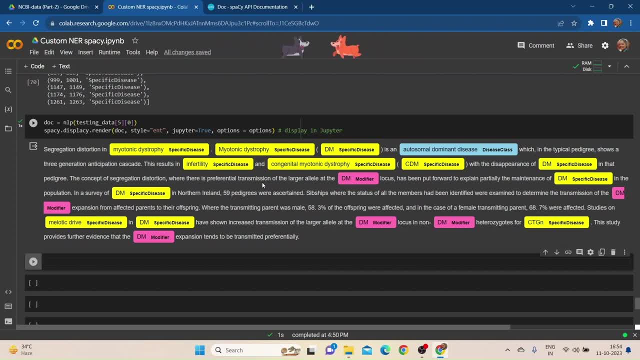 And as technology continues to advance, NER will surely play an increasingly important role in our daily lives. So if you need any kind of implementation of NER, Or if you want to discuss more about this implementation, Then please feel free to contact us. 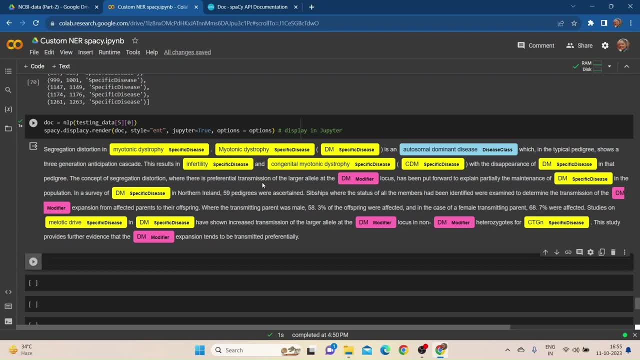 We will try to help you to the best of our abilities And if you have made it so far into the video, Then thank you for joining us today Into this journey into Named Entity Recognition. We hope you have gained a better understanding of this powerful NLP technique. 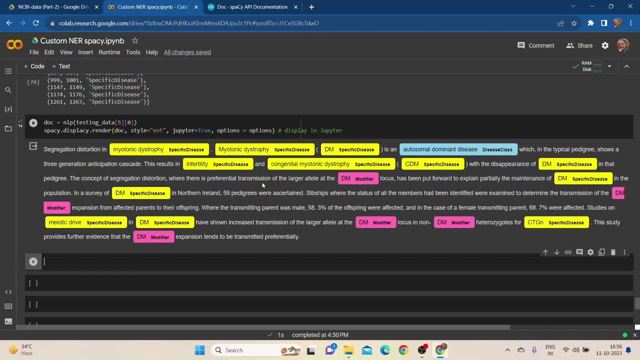 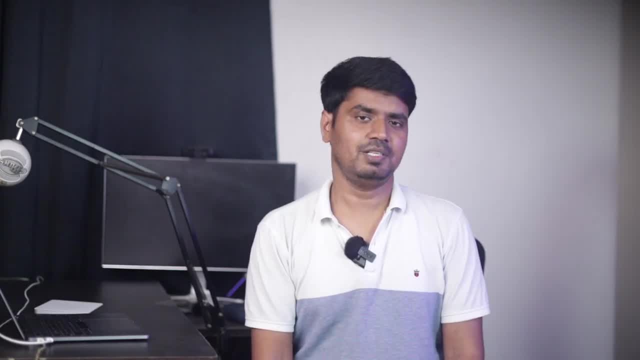 And I request you to stay tuned for more such exciting projects and topics. Thank you, So that's all everyone. I think you enjoy the video And you get some insight from this, And maybe you hope you learn something Even more. This is as a final note. 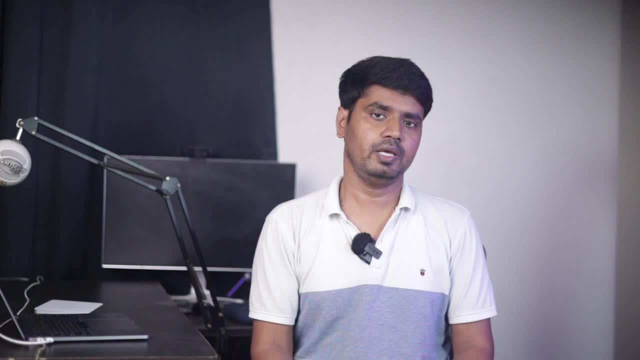 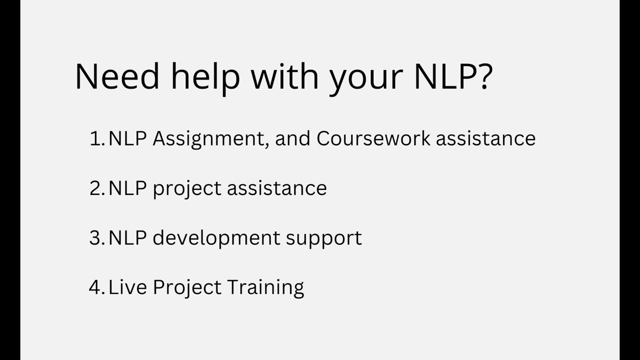 So if you are working on this type of projects, Or even you need any projects, Either in any type of task- Like NLP task, Like might be it's assignment Projects, Course work And even development- in We offer a variety of services. 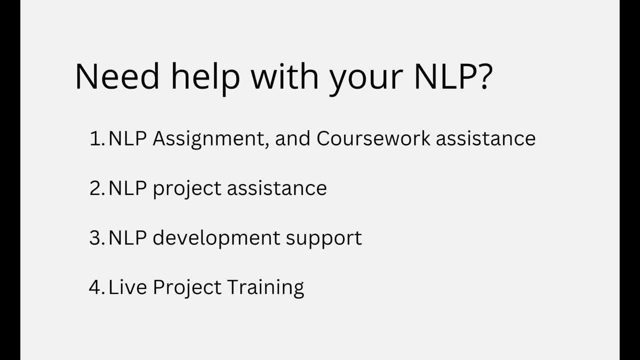 To help you And get your job And get your job done. So just a normal on demand, On demand services Like NLP, assignment assistance. So generally this type of services are requested by a student Or developer who are just a learner. 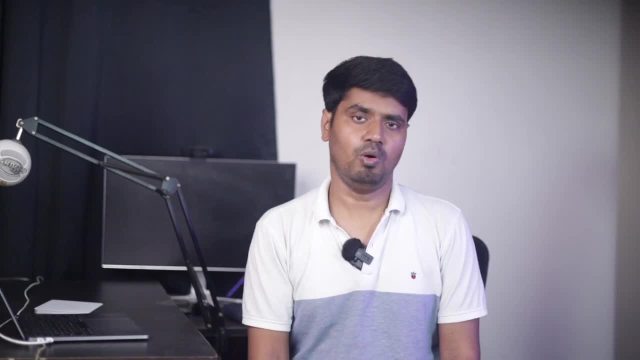 So in this type of projects, We can help all the aspect of this project, From research, Data collections, Analyzing, Reporting And code implementation. As a project developer, We can help you With development assistance. We help to All the aspect of your projects. 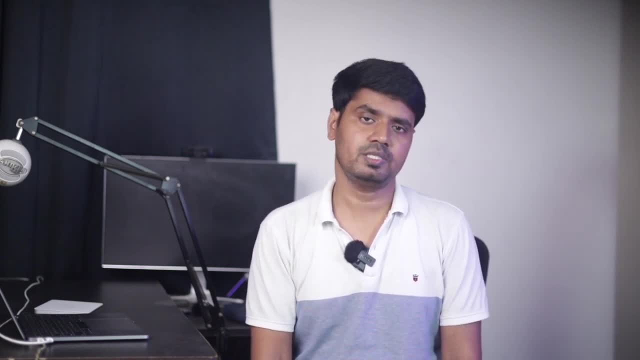 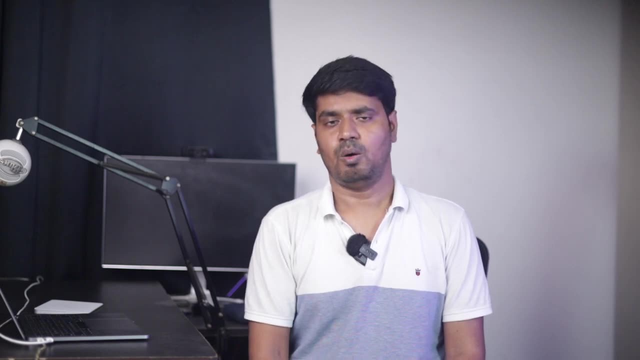 Like planning, Development, Implementation And even the maintenance phase, And during the need, More and more resources To complete your project on the time, As we want to launch, Moreover, Like as a startup And others company, Hire us. 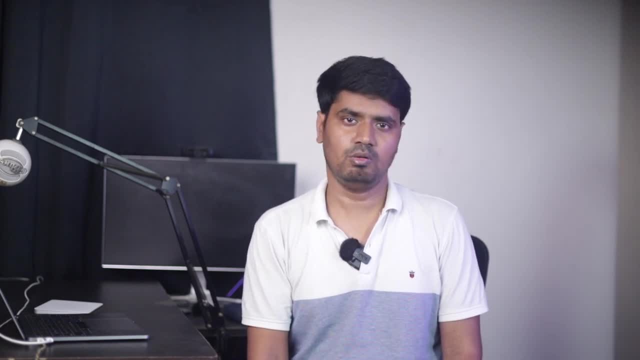 For their development support. We can also provide All the expertise You need in AI ML domain. More specifically about this project, So NLP Or NIR related, We can help to develop your Own NLP solution Based on your need. 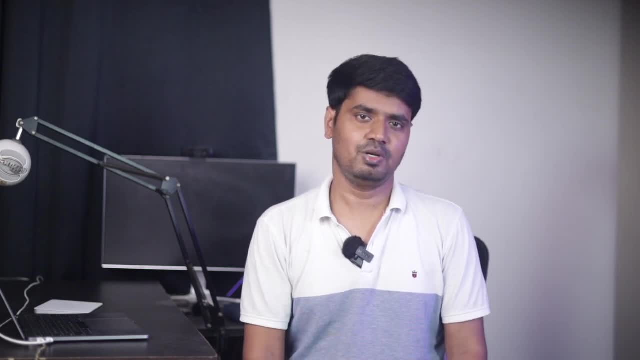 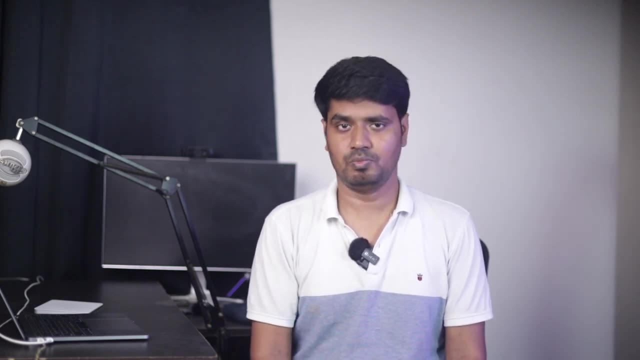 On the demand. Okay, And the final one is, You know, Launching your own product. So app development. So if you are building your own Custom NLP application, Then you can surely Check out our website. And what are the different.